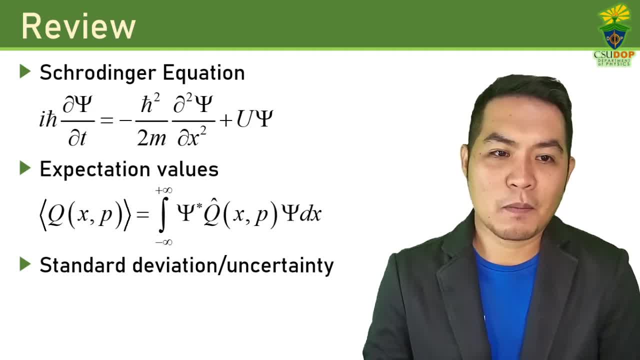 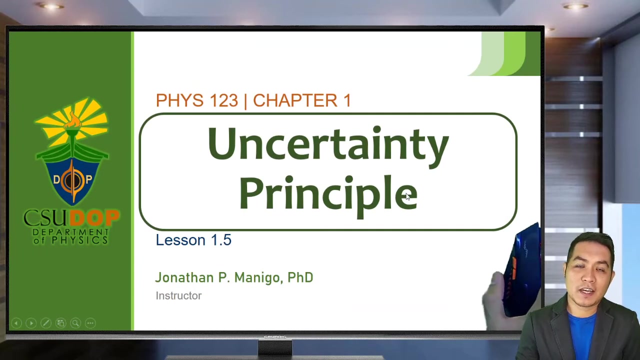 We also have discussed in the previous lessons about standard deviation, which represents uncertainty, And we will relate that to our last topic for this session, which is all about The Uncertainty Principle. So you may have discussed the basics of uncertainty principle in your modern physics, which 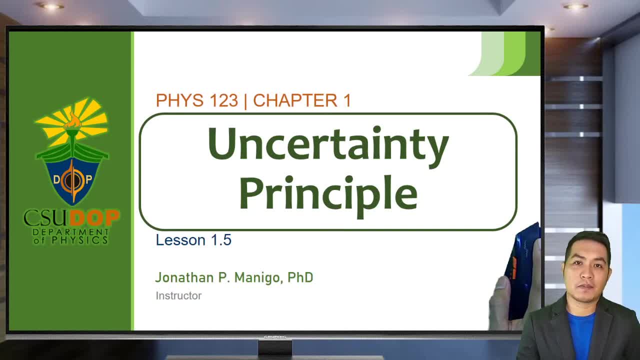 maybe one uncertainty principle that you have discussed is the uncertainty between position and momentum, and we will focus with that in this chapter. so we will generalize: we will not be deriving the uncertainty principle in this lesson. instead, we will derive the generalized uncertainty principle when we formalize the discussion of quantum mechanics in chapter 3. so let's. 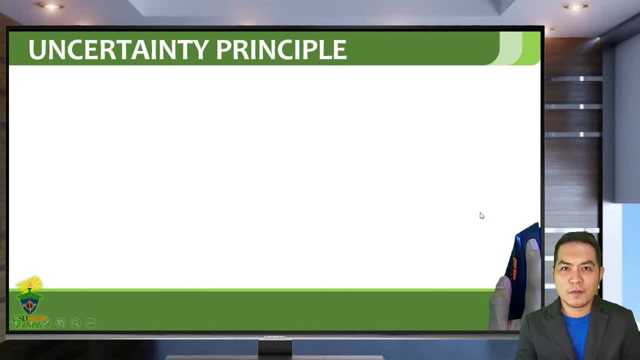 start our discussion with position and momentum: quantum position and quantum momentum. so, for instance, your probability density, absolute value of your wave function squared, or absolute value of your wave function squared, is the value of psi squared. probability density will looks like this: so, in this example, your position is indeterminate or undefined, because there are many 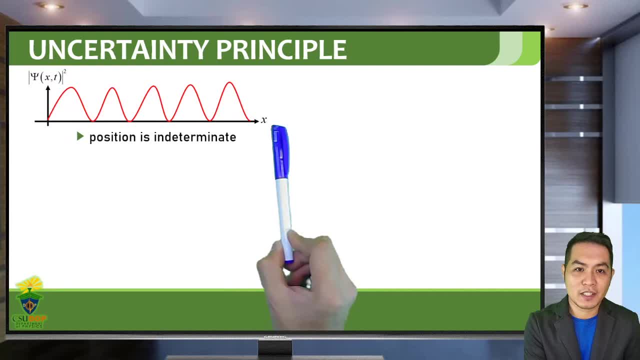 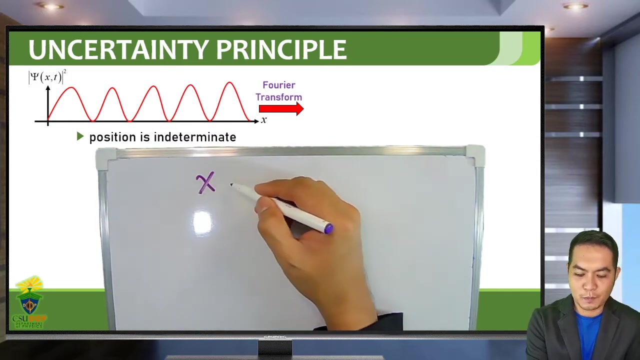 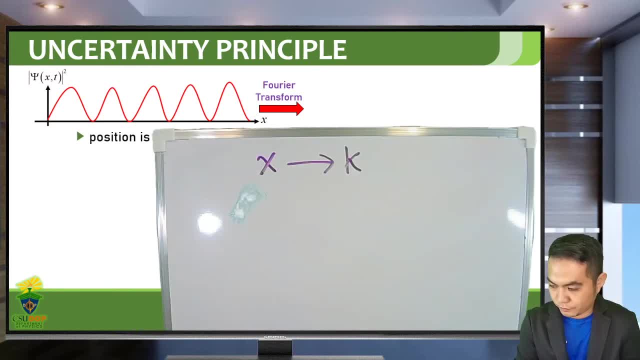 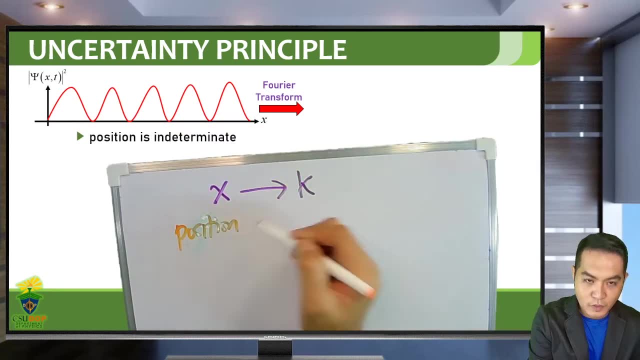 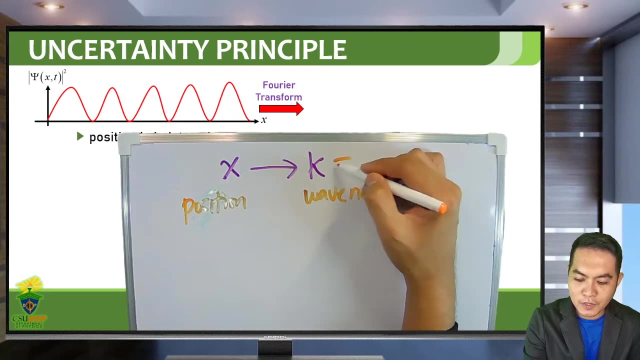 X is position. okay, is what we call the wave number. it's actually equal to two pi over lambda. X has a position of length, say meters K has a position, sorry K has a unit. X has a position of length, meters K has a position of. sorry K has a. 하다. X hata positi 마 location sa metum. I pata ma 2 pi错. it's a wentat. x has a position of样 meter's, K has a unit. x has a position of church by position of k. but ah, Sorry, prove it again. k has a unit, x has. 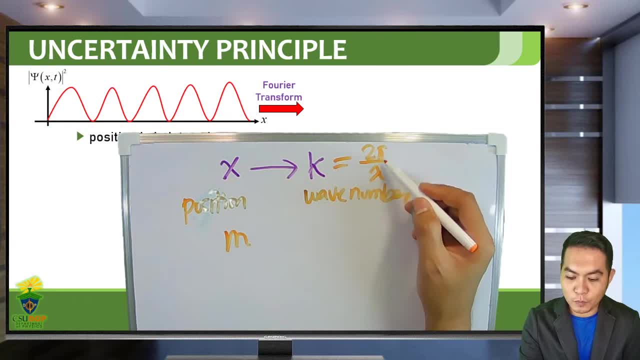 of length or meter. k has a position of 2 pi over lambda, so 1 over length or say 1 over meter or meter inverse. so this is the in, this in. in your solid state physics you usually call the k-space as the reciprocal space, because the units 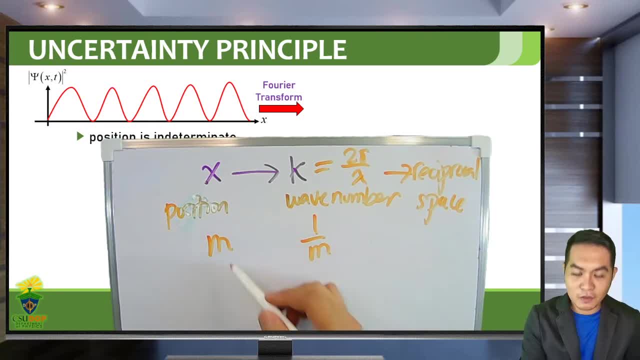 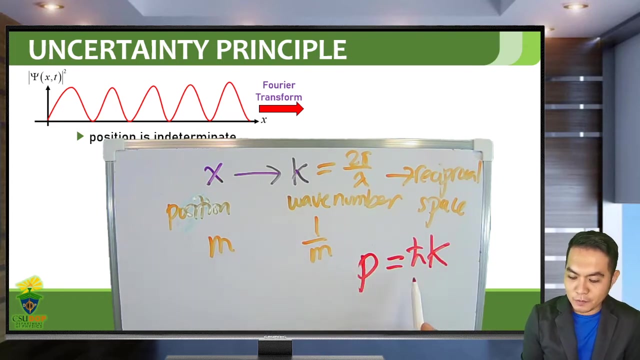 in that space are reciprocal of length. reciprocal length, so reciprocal of position. so in your modern physics you have discussed about the quantum mechanical result of momentum, where in momentum is just h-bar times k, so meaning, since h-bar is just a constant, if you multiply your wave number by 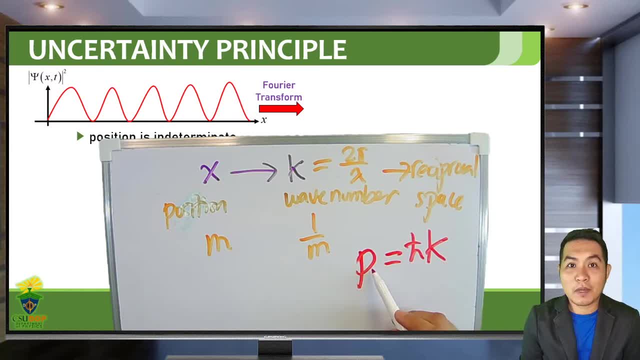 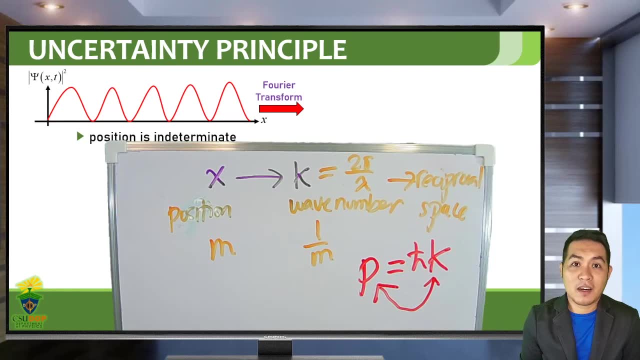 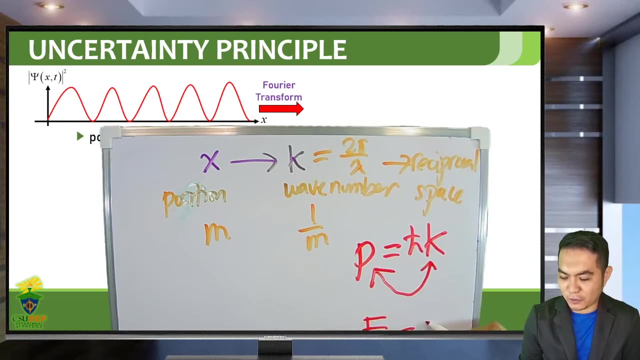 h-bar by a constant h-bar, then that on that becomes the momentum. so essentially k and p, k and momentum are the same because they're just related by a, by a constant similar when we say, energy is just equal to mass, because they are just related to a constant c squared. so energy is just essentially mass. so here, 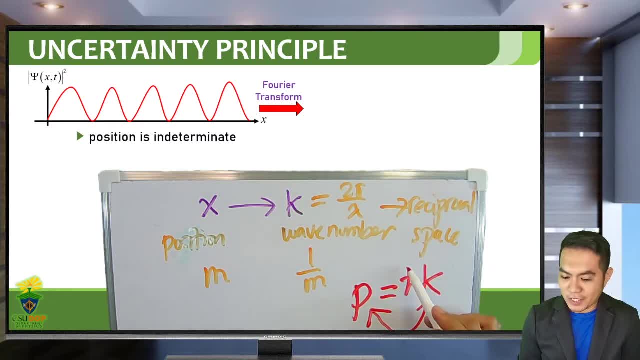 momentum is essentially wave number, which they're just related by a constant h-bar. so when you fully transform to the k-space is actually just transforming to the momentum space, because you just multiply your k values by h-bar and they become momentum. so when you fully transform this wave function, 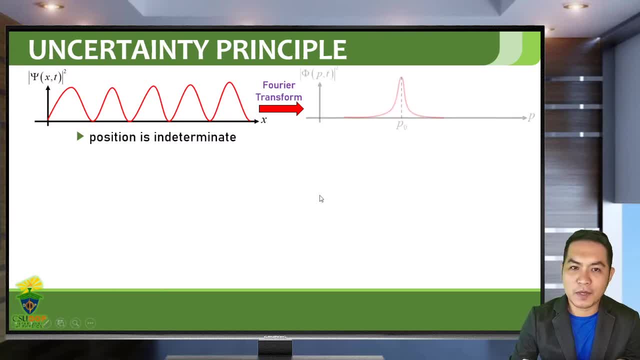 probability distribution, psi, squared into the momentum space. it will look like this: your momentum, your wave function now is now momentum space wave function as a function of momentum and p and t, and it will look like this: the momentum will now be become defined, so you can actually think of this as a wave. this is a wave. 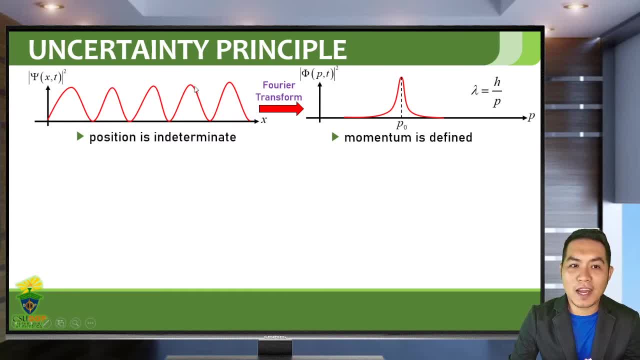 right. so a wave has a wavelength lambda. so if you have a wavelength lambda, then based on de Broglie's hypothesis, then if you know the wavelength, the quantum wavelength, for for that matter, then you will know the quantum momentum. so here you don't know the position, but you know the wavelength, so you know the. 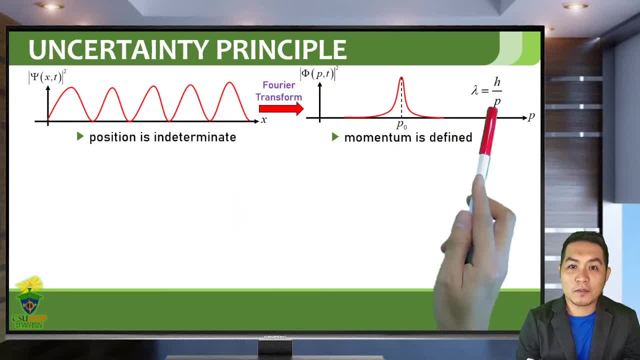 you know, the quantum momentum or the momentum is defined, conversely, if you're a position space wave function, psi, as a function of x and t squared, the probability distribution will look like this: it's defined for a certain value of x, say x-naught. so usually this happens when you measure the position of the 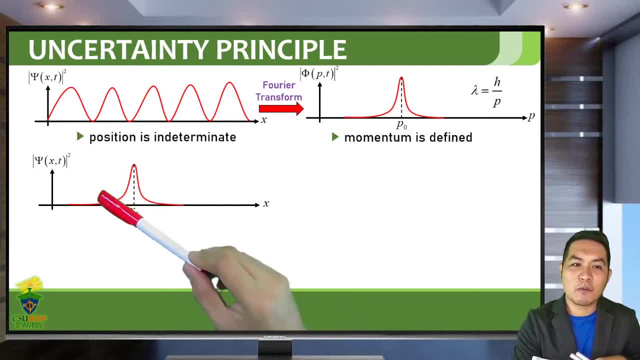 particle. so when you measure the position of the particle, you know the measure, the position of the particle. the wave function actually collapses into one, into into in, or close to one value of X, such that the particle takes a stand, or you're actually confining the particle to one position, that's. 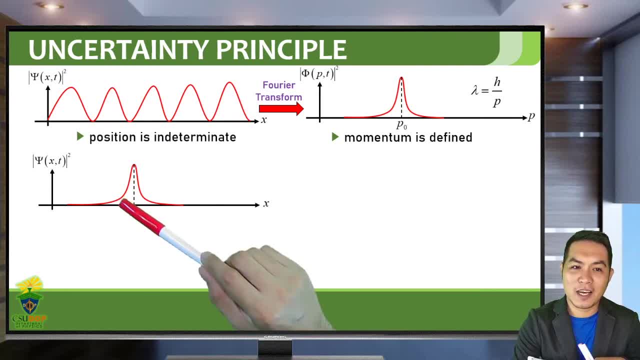 actually what measurement in the quantum world is all about. so when you, when you measure the position of the particle accurately, when you transform that into into the Fourier space, so you measure the position, you define the position if you transform that in the momentum space, so in the momentum space, this axis is now momentum. so you will notice that you no. 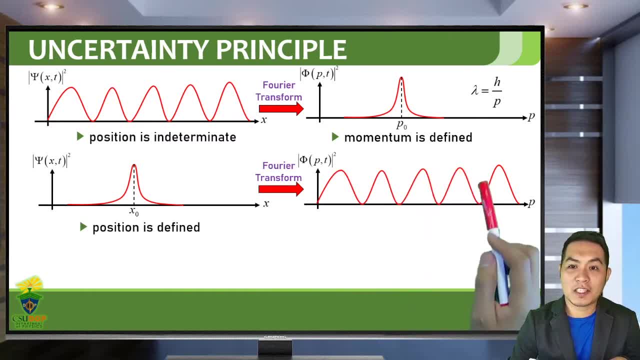 longer know what is the momentum of your particle. so the move, the momentum becomes indeterminate or indeterminate, undefined. so that's actually what what is Heisenberg uncertity principle is all about. so it states that you cannot measure position and momentum at the same time. so if you measure momentum, you lose information about its. if you, if 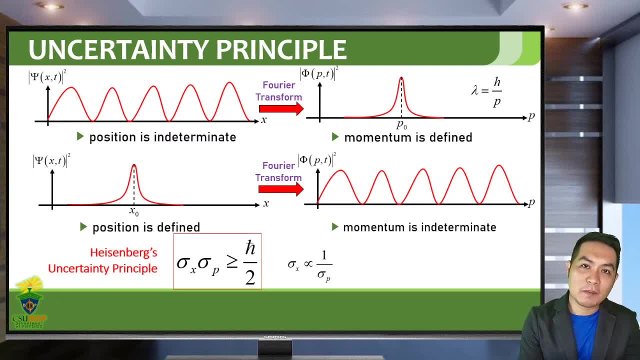 you measure the momentum of a particle, you lose information about your position. conversely, if you measure the position of the particle, you lose information about its momentum. so there's just a limit to what you can measure simultaneously in the quantum world. so most variables in the quantum 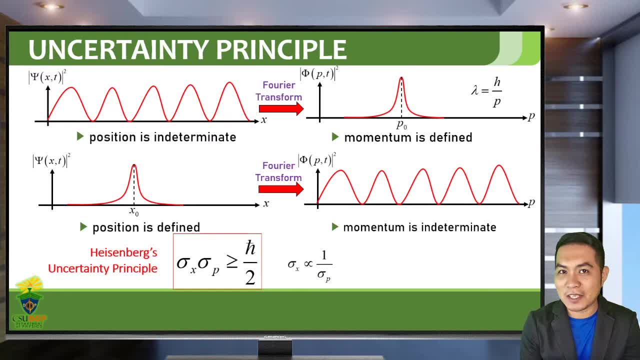 world cannot be measured simultaneously, but of course there are variables with which we can measure simultaneously, and we will discuss that in the future chapters. so this is the mathematical form of Heisenberg's uncertainty principle. the standard deviation or the uncertainty in X multiplied by the standard deviation or uncertainty in P in momentum must be greater than or. 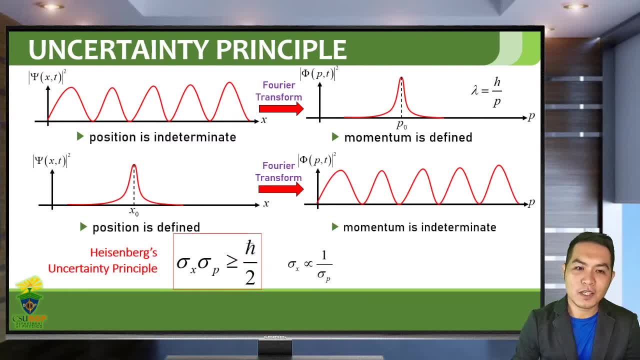 equal to each bar over 2. so this is the limit. so you will notice that each bar, each bar is the Planck's constant. it has a in the orders of magnitude of 10 to the negative 34. in the classical realm, H bar is actually very. 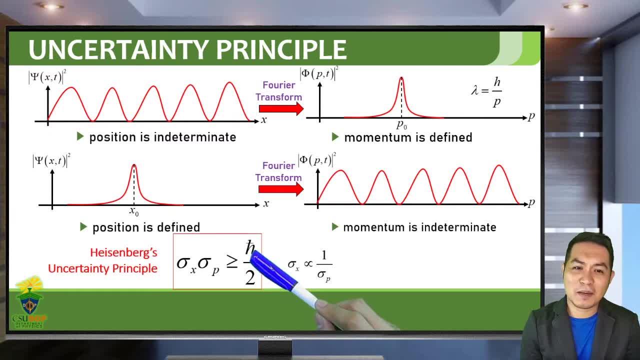 very small: 10 to the power of negative 34. that's a very small number. so in the classical realm this is actually equal to 0, which means in a classical realm you can simultaneously measure position and momentum at the same time. but in the quantum realm, in the realm of very small objects, even though each of our extent to the 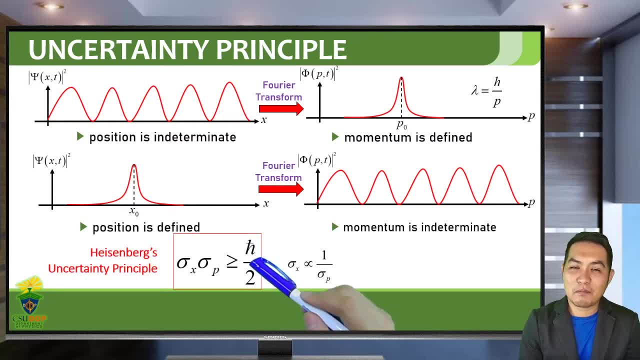 34, but each bar is a big number when it comes to the quantum world, so that is why this is significant. in the quantum world, do the H bar, but when you go to the classical realm, each bar is actually a very small number, so it's approximately equal to zeros, so meaning you can measure both position and 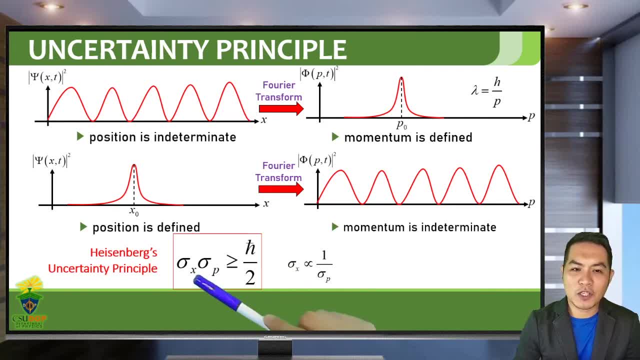 momentum at the same time. so if you rearrange the equation, you will notice the relationship between the two uncertainties. they're actually inversely proportional with each other. so that is, that is what I have been telling earlier, that if the uncertainty in X is very small, meaning very small. 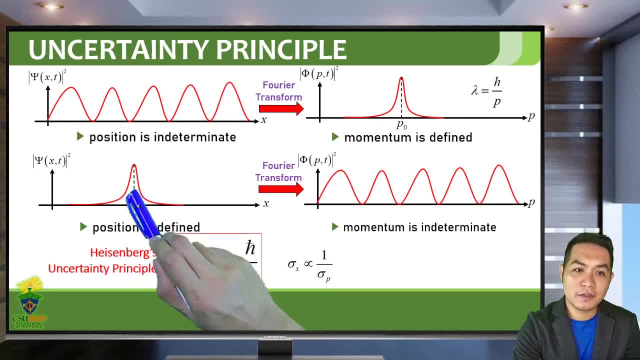 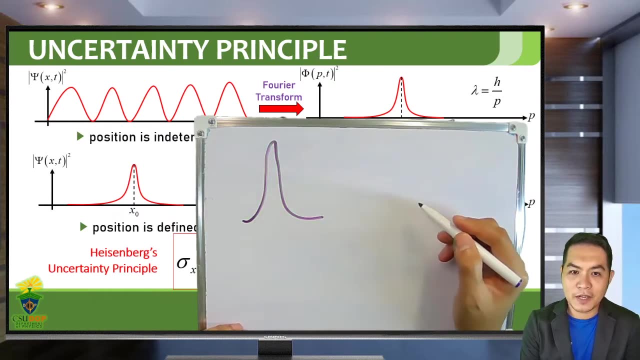 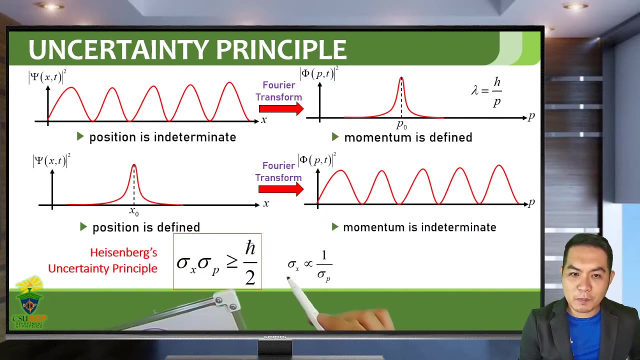 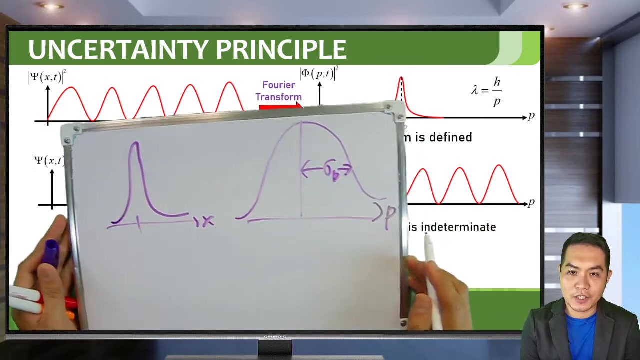 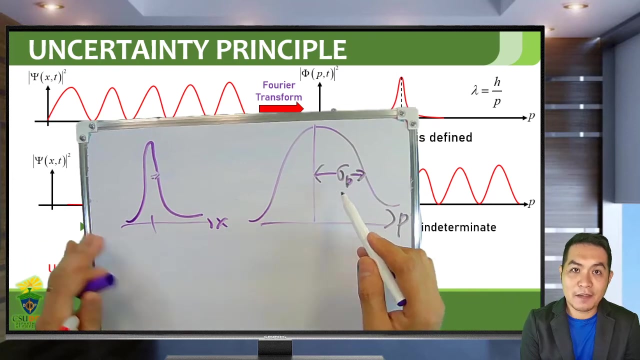 standard deviation very small, spread from the mean. so so say your position is defined. very small standard deviation in X. then your momentum, since they are inversely proportional, then the uncertain uncertainty in momentum will be large. so small Sigma X will correspond to a large Sigma P, and inversely, if you have a large 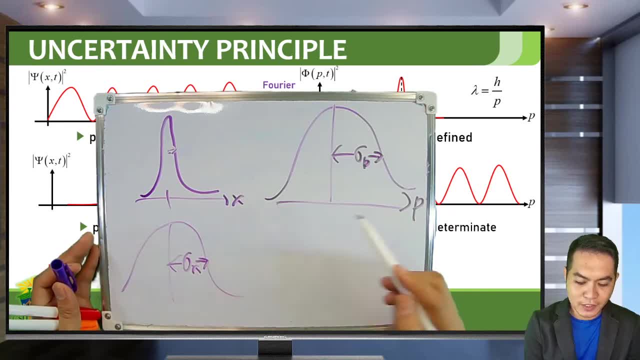 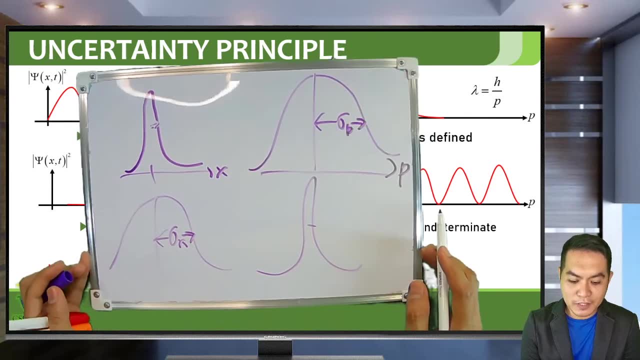 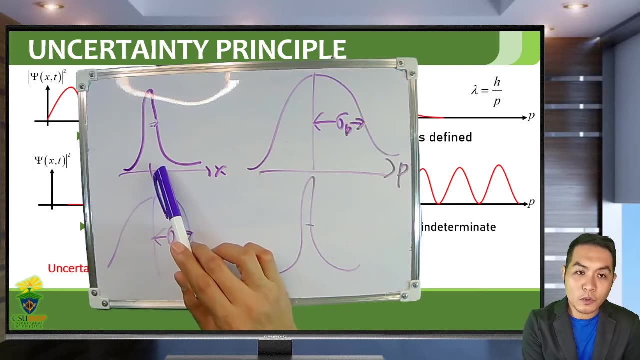 Sigma X, large uncertainty in X, then you will have a small uncertainty in momentum's there's. they are inversely extraordinarily so, meaning if you have, if you'd know, if you, if your position is accurate, your momentum will not be accurate. if your position is not accurate, your momentum will be accurate. so that's what high, simple uncertainty principal is all about, as described by Heisenberg, If your position is coincidentally accurate, then you are doing a very high level up roller. If your momentum is invisibly accurate, If the slower movement is Uranus, the largestizing momentum in Earth, is always an active number, for which your Despotefirppe's- So you are always density or moment- will be active for your faced-���lass ballet with your momentum is arie. Vous are always apparent in your cleansing line last Sch prosecco, because what you can get if 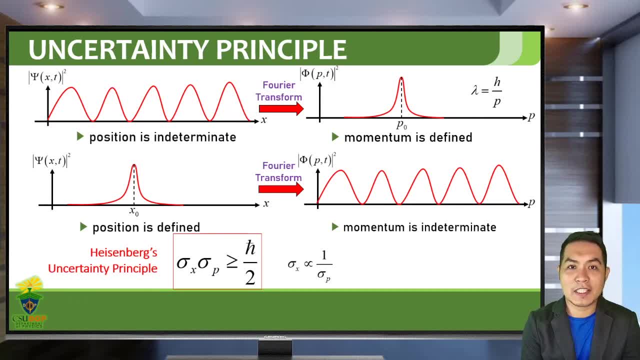 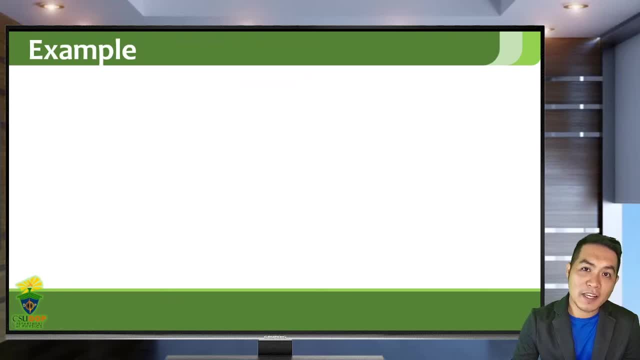 all about. okay, so this will be the last topic for this chapter. so for our example, we will have- will now have- an example which will incorporate all of the lessons that we have discussed so far for this chapter. so this problem is like the generic, the complete problem for this chapter. so, suppose you? 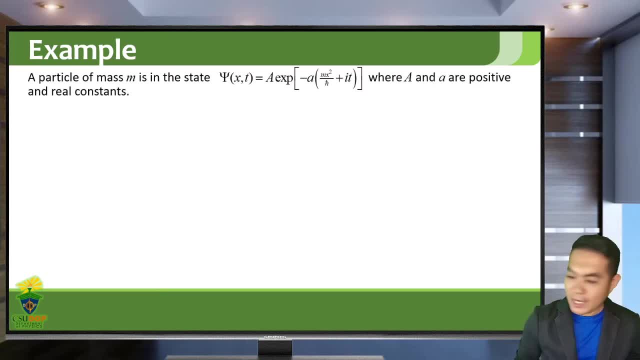 have a particle of mass M and it is in the state given by this wave function. so notice that our wave function here is now a function of X and T. there's now a time component, so we're capital A and small a are positive, real constants. so you are asked to find a, the normalization constant. so you: 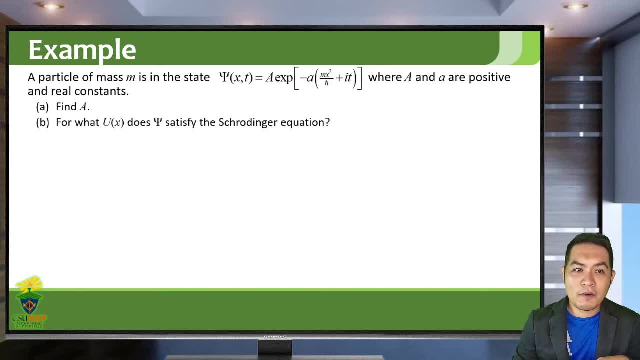 normalize your wave function. so for what wave function? sorry, for what potential energy? you, as a function of X, does this wave function satisfy the Schrodinger equation. so what's the potential energy if your particle is in this state? so you need to use the Schrodinger equation for letter B and 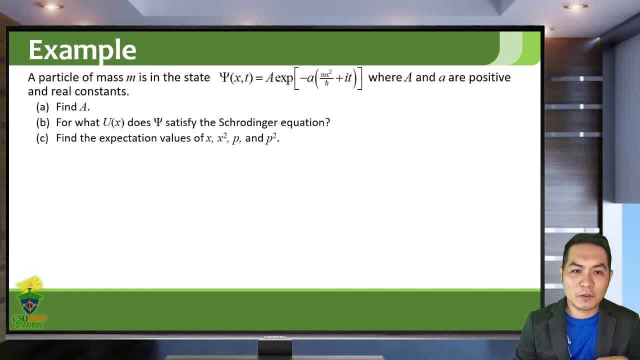 you are asked to find the expectation value of X, X squared, P and P squared. so, of course, if you know the expectation value of X and X squared, you can find the uncertainty or standard deviation in X. if you know the uncertainty- sorry, the expectation value of P and P squared, then you know the standard deviation P. 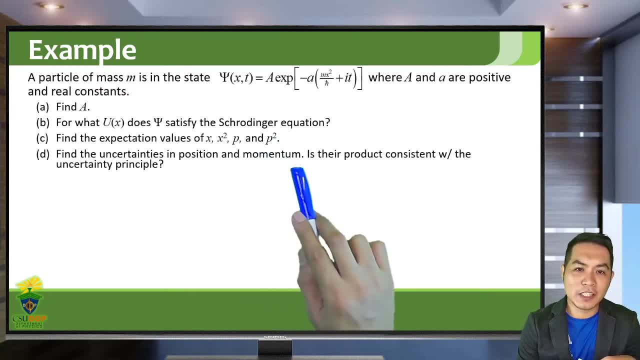 or the uncertainty in P. so you find that in letter D and check for the consistency of the uncertainty principle. the uncertainty principle is not the answer, but the answer is the uncertainty principle. and that's why we have to go through the problem before we can actually violate the uncertainty principle or not. okay, 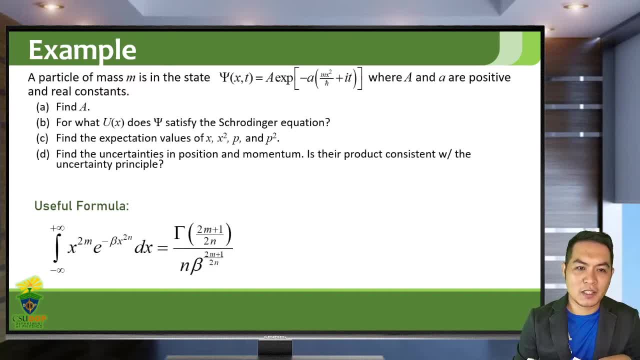 for this problem there will be a useful formula. actually, this is a very useful formula in this chapter, in the next succision chapter. this is sometimes called the Gaussian integral formula. so if you encounter an integral like this where M and N are integers and it can start from zero, zero, one, two, three, four, 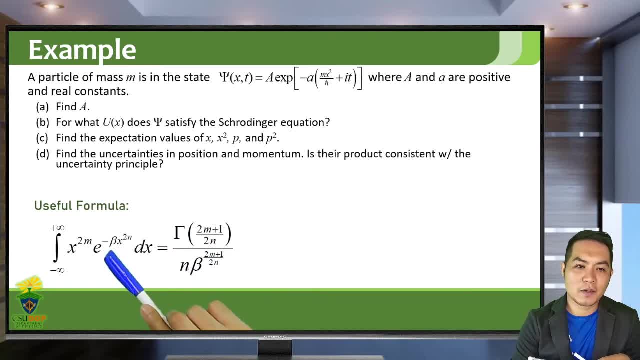 n plus 1 over 2n times n beta- where beta is just a constant here- to the power of 2n plus 1 over 2n. again we have discussed about the gamma function. it's just related to the factorial function and the gamma of one half is actually square root of pi. so using this relation, gamma of v plus 1. 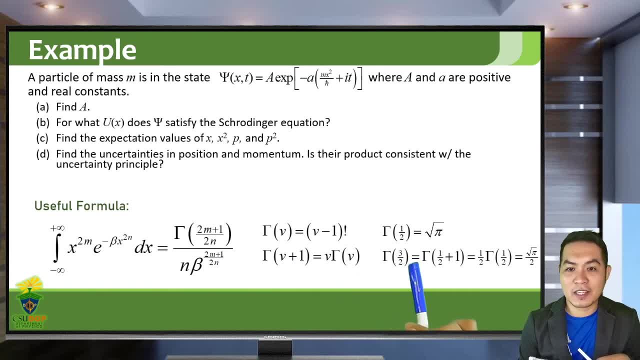 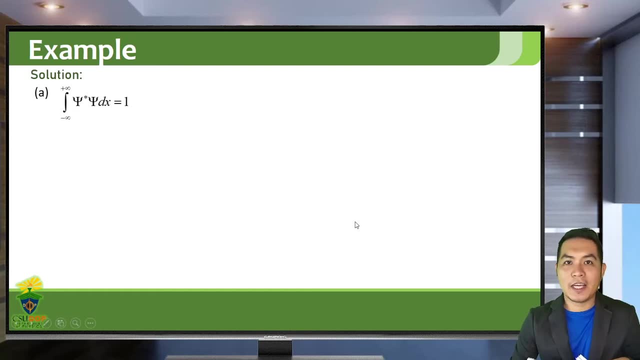 is equal to v, gamma of v. the gamma of three halves is essentially gamma of one half plus one, so it's just one half gamma of one half, or square root of pi over 2. okay, so for the first problem we are asked to find a, the normalization constant, so we use the normalization condition. so instead of 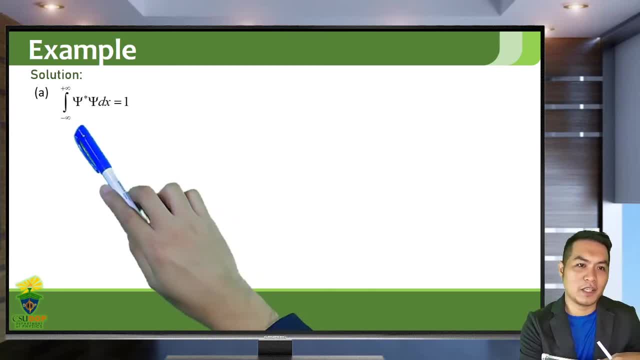 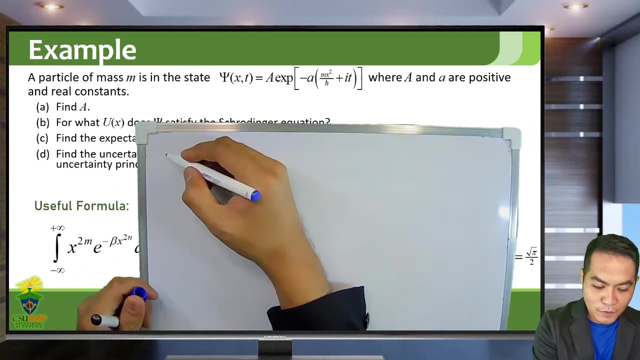 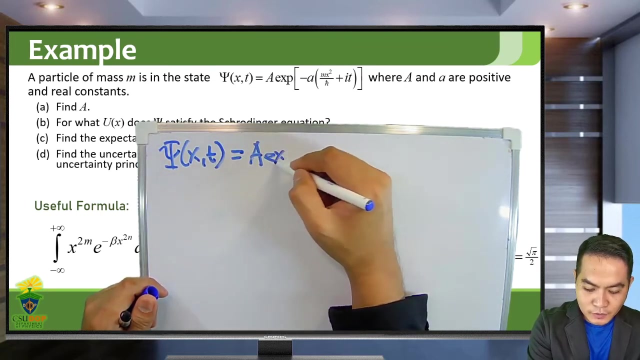 using absolute value of psi squared. here we use the more general form of absolute value of psi, which is psi, star psi, you okay, sorry, so let me just uh, i forgot to place the wave function here, so let me just copy our wave function: psi as a function of x and t. it's a exponent of negative a mx squared over h bar. 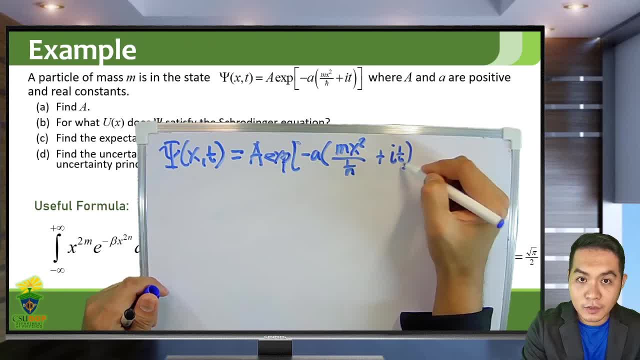 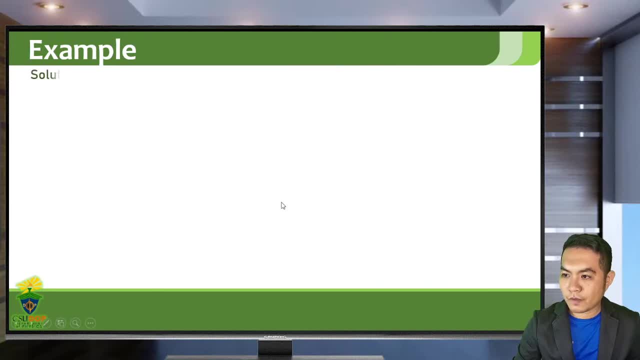 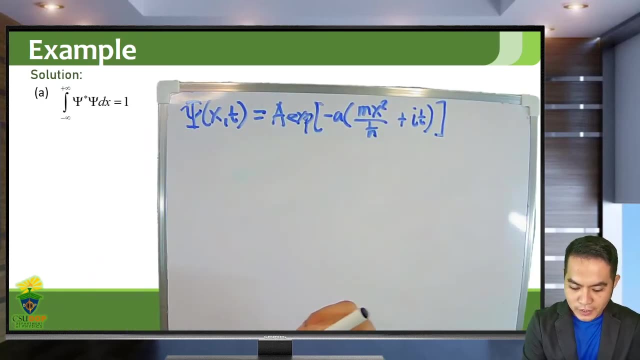 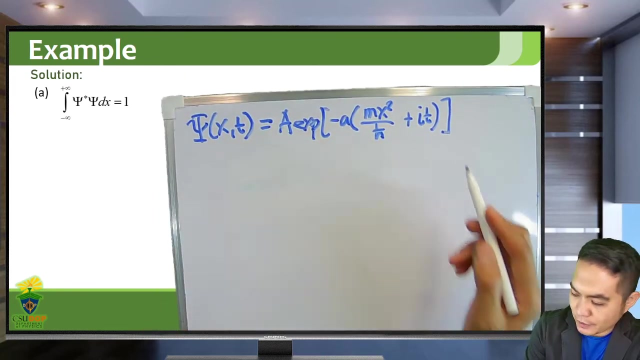 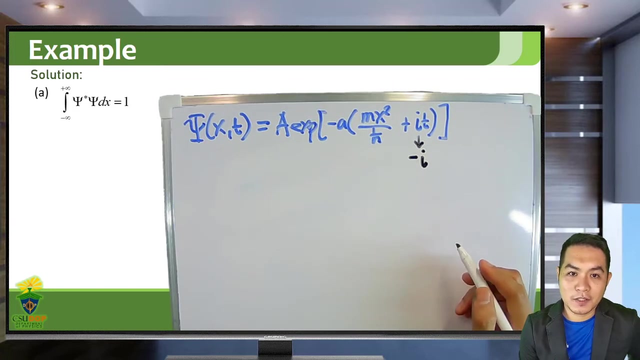 plus i t. okay, so this is our wave function. okay, so we use the normalization condition. so we take the integral of the conjugate of this, so you have i. so when you take the conjugate, this becomes negative. i, we take the conjugate, so you will. 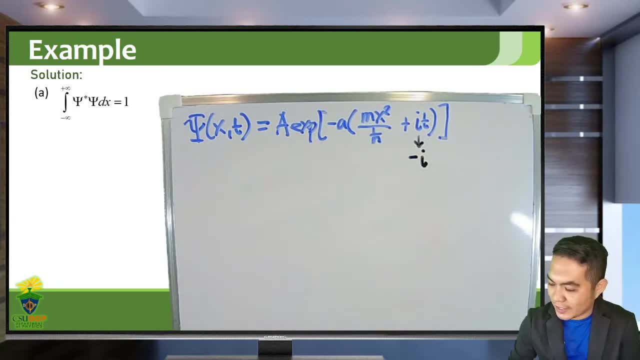 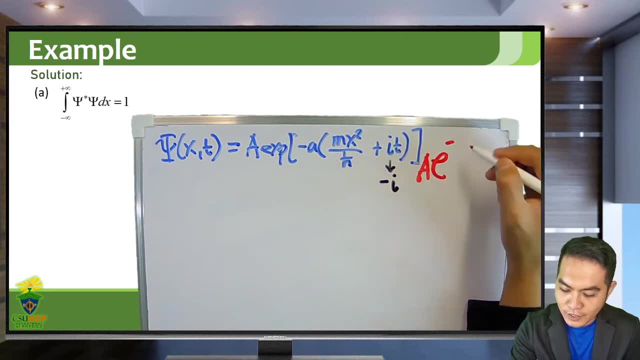 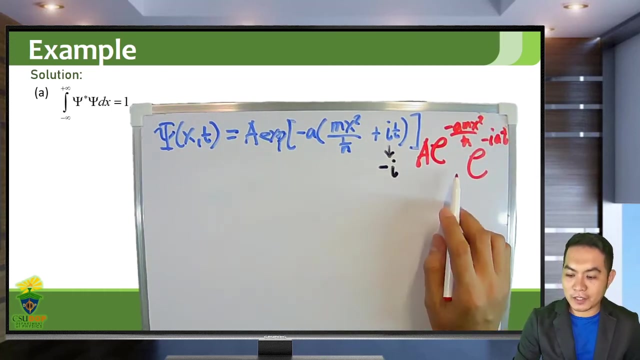 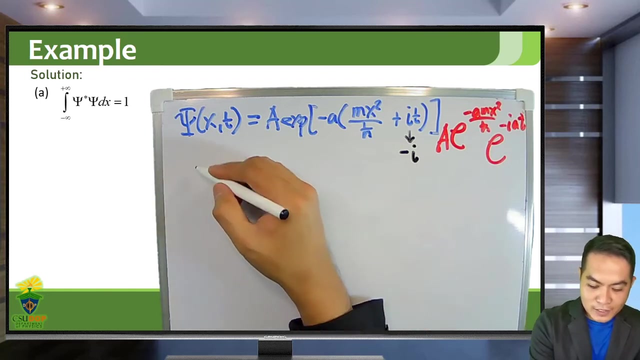 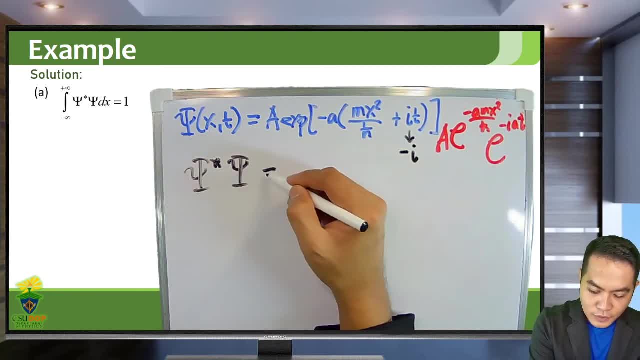 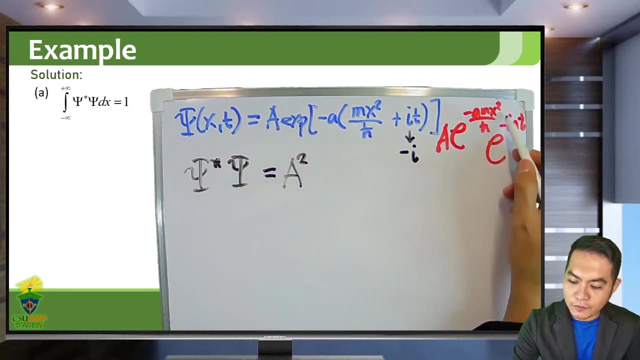 psi, star psi, you will notice that, uh, since this is a real, then it's conjugate, it's just itself. so it's just a squared. so also the first exponential is also real. there's no imaginary here, so it's just conjugate, it's conjugates itself. so 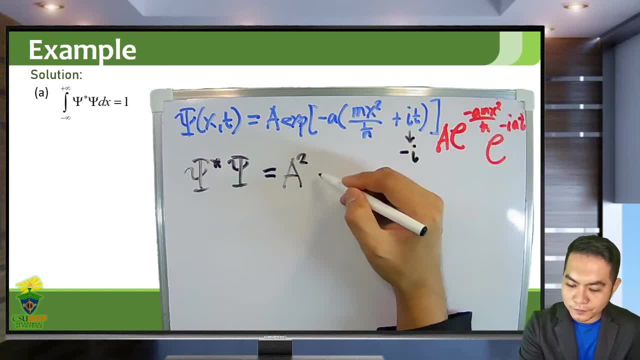 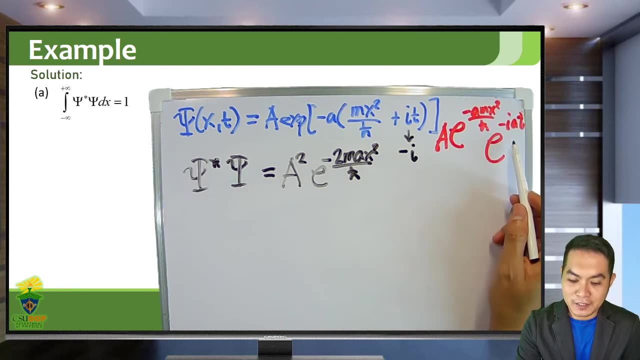 psi star times psi is just the square of that one. so you will have e to the negative 2, say m a x squared over h bar. but here the conjugate of this exponential term is e to the positive i a t and its original form is e to the negative i a t. so you multiply those two- e to the i a t times e to the negative i a t- and you will get e to the zero or one. so 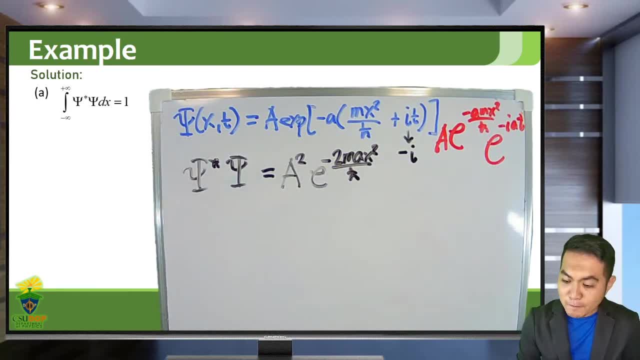 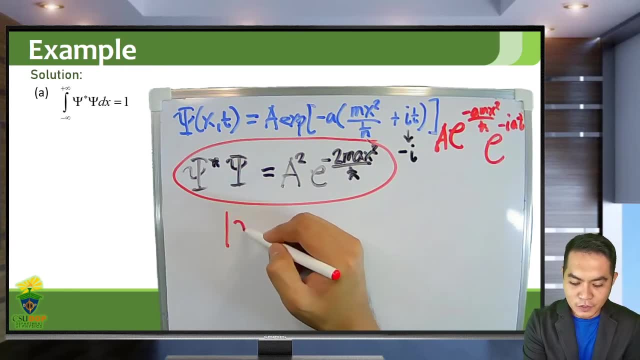 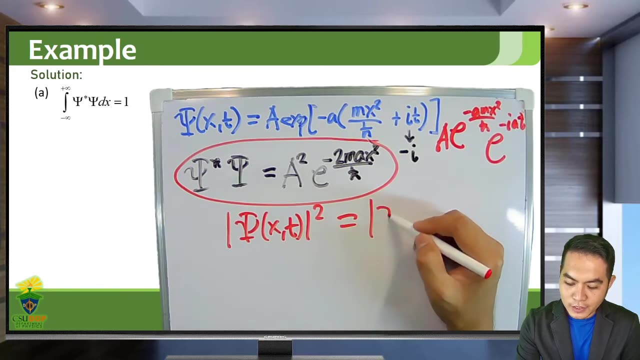 that's it. in this case the time component will actually cancel each other out. so also in most of our examples, when you take the absolute value of psi squared, where psi is a function of x and t, it now only becomes a function only of x. the time component most of the time cancels each other out. but note that this is not a general. 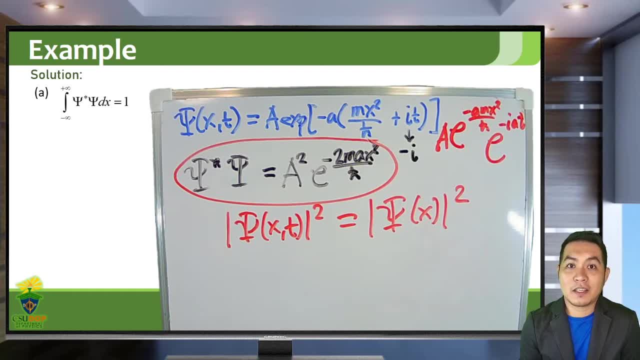 situation. it's just there. there are still some examples when you take the probability density, and it's still time dependent. so for this case, this is truth. for our example. okay. so this is our absolute value of psi and it's still time dependent. so for this case, this is true for our example, okay. so 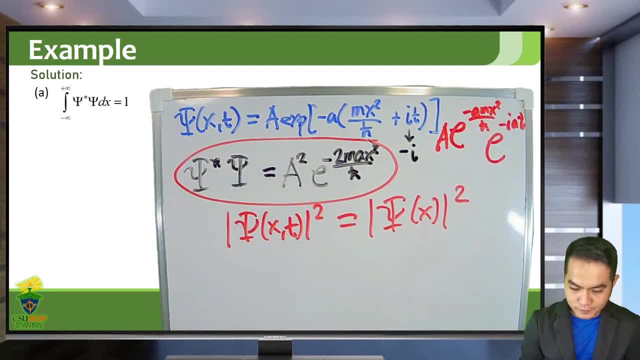 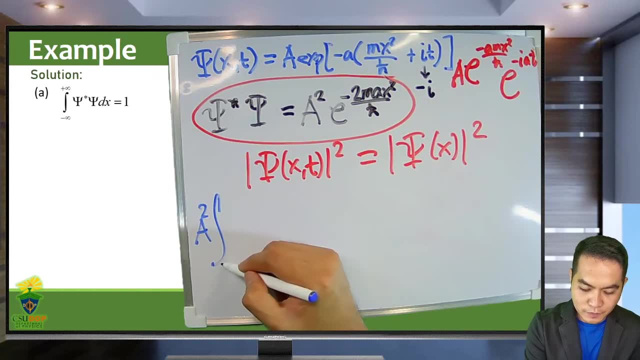 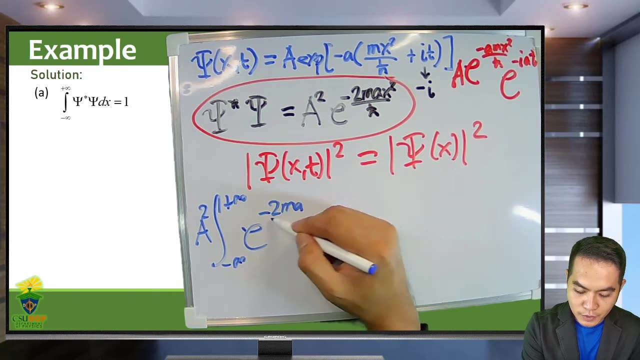 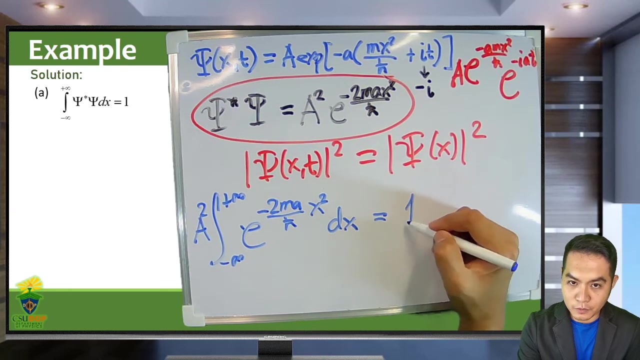 so values to And in our integral you will get- So I will take out the video- a squared from negative A, what finished a I, what AT positive infinity of e to the negative 2 ma over h, bar x squared dx, and it should be equal to 1. okay, so I will go back to our integral formula, our Gaussian. 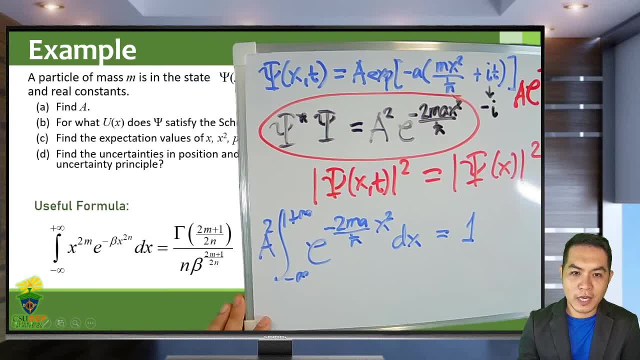 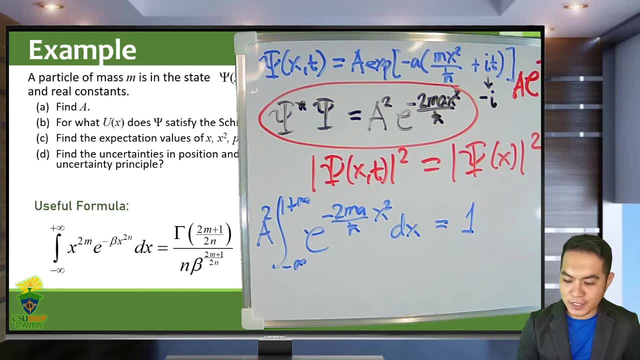 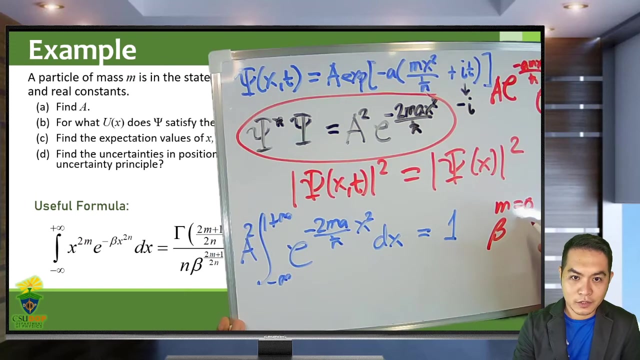 integral formula, which is this one, and compare. so we will use this formula and by comparison we see that M is equal to 0 because there's no X here, so meaning M is equal to 0, X to the 0 is 1 and in this case our beta is 2. ma over h bar. 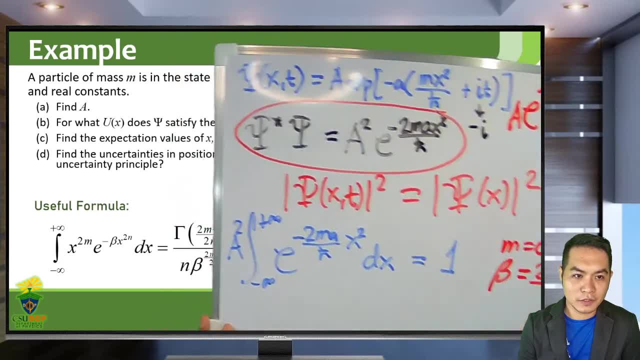 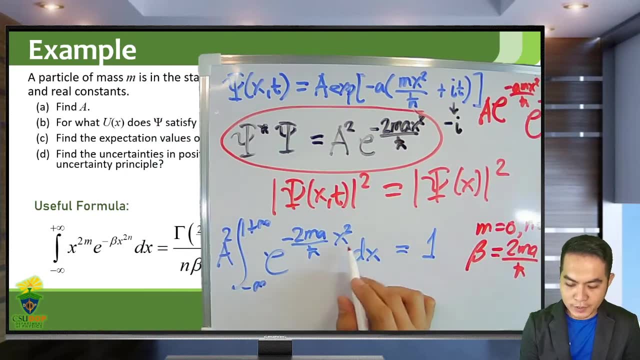 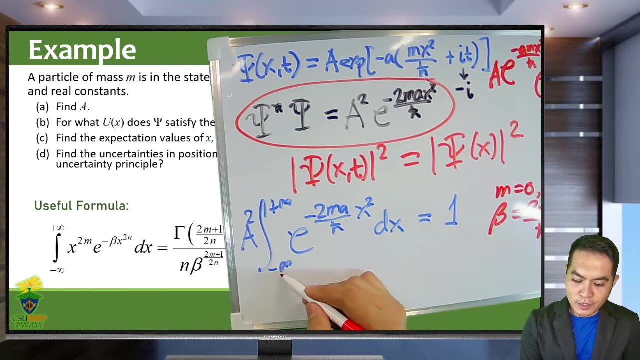 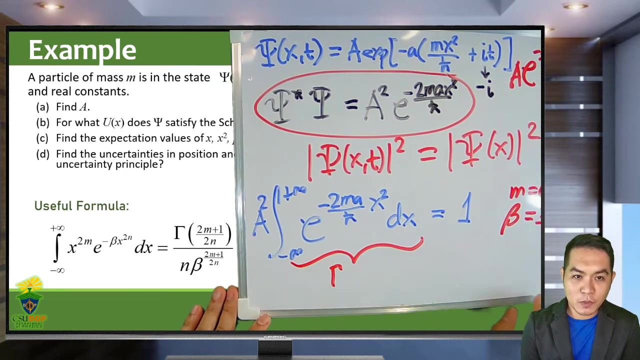 and this is our beta and our M is equal to. so this is X squared, this X to the 2 and meaning n is equal to 1. so therefore, based on the formula, this integral is just gamma of 2m plus 1 over 2m. so M is 0, meaning 0 plus 1, so 1 gamma 1 over 2n. 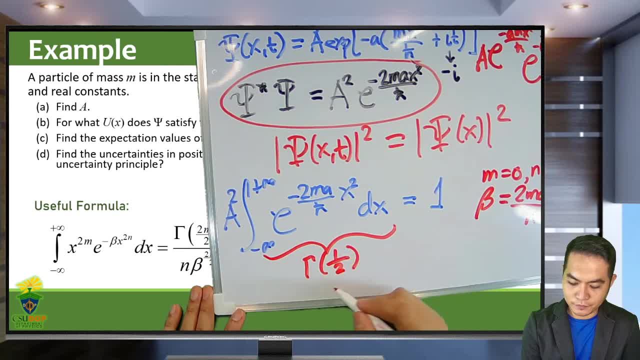 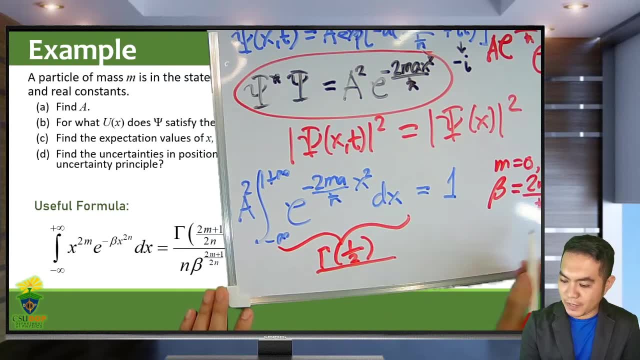 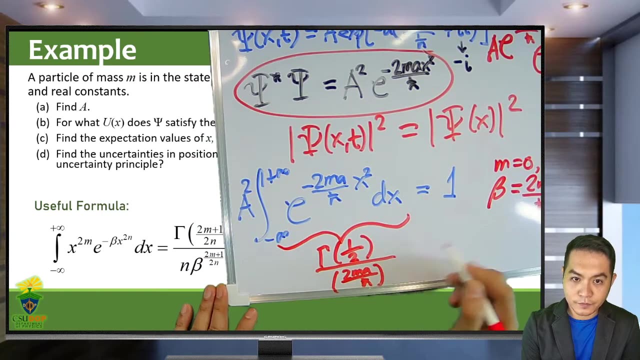 and is equal to 1. so gamma 1, half all over beta, which so n is just equal to 1. so n is just equal to 1 and beta is this one 2ma over h bar, so 2ma over h bar to the. 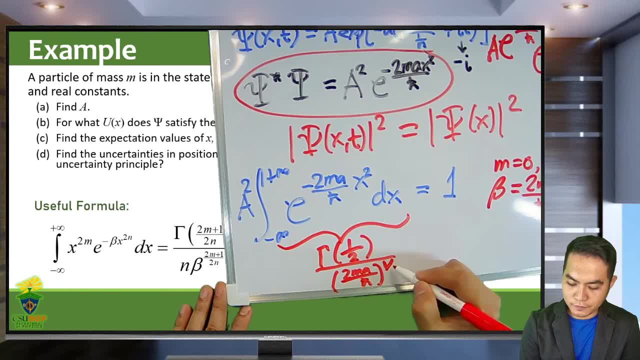 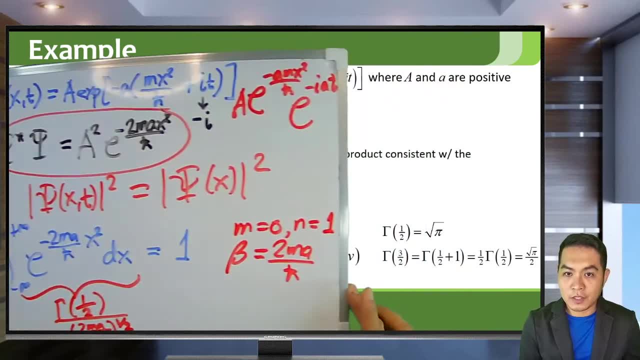 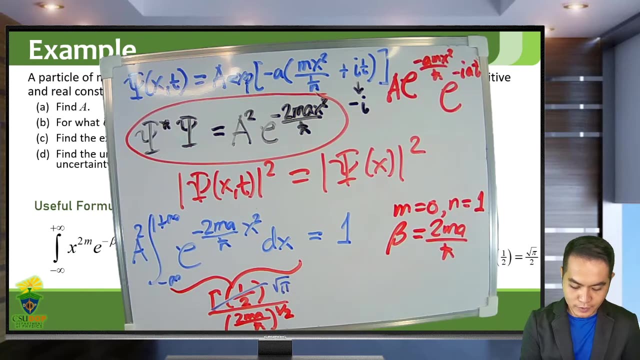 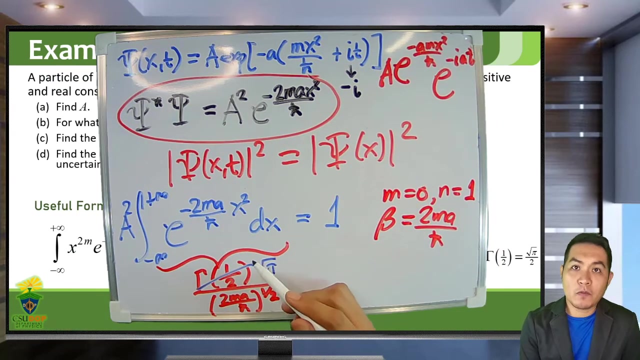 power of this one 1 half. okay, so gamma 1: 1, 1 half is just this one square root of pi. so this is just actually equivalent to the square root of pi. so simplifying, since we have already evaluated the integral, simplify so you get a squared is: 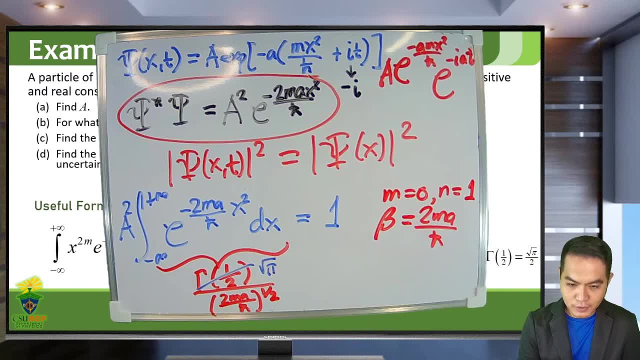 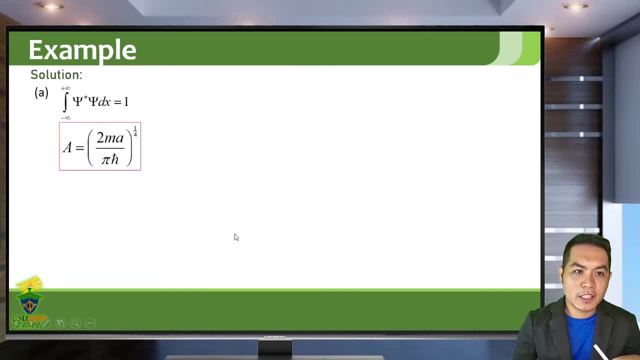 something like equal to some value. you take the square root and you will get this value here. so a is equal to the fourth root, 2ma over pi, h bar to the power of one fourth. so our wave function will now look like this. so we replace our normalization constant. 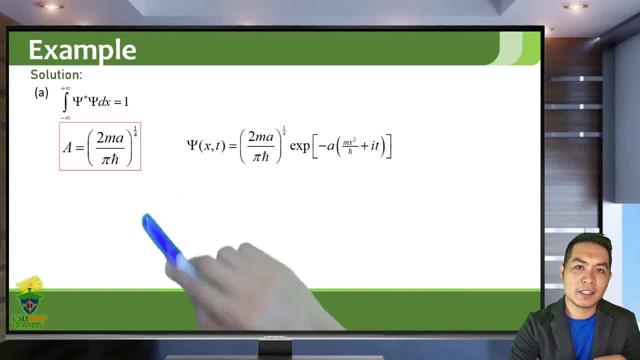 a with the value that we have obtained here. okay, second question: for what potential energy does our wave function do satisfy the schrodinger equation? so recall, we recall our schrodinger equation, so we actually know the form of psi. psi is known, it's a function of x and t. uh, the only unknown, actually, in our 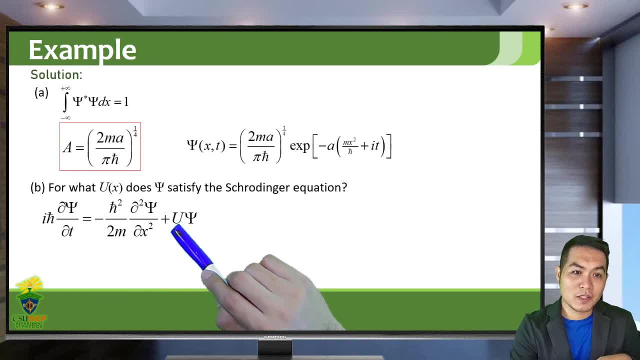 equation is u, so essentially, we solve for u, given our psi. so therefore, we need to find partial of psi with respect to t and the second second partial derivative of psi with respect to x, and then solve for u. that's what we will do for this problem, or that's how we solve this problem. so, given our psi, 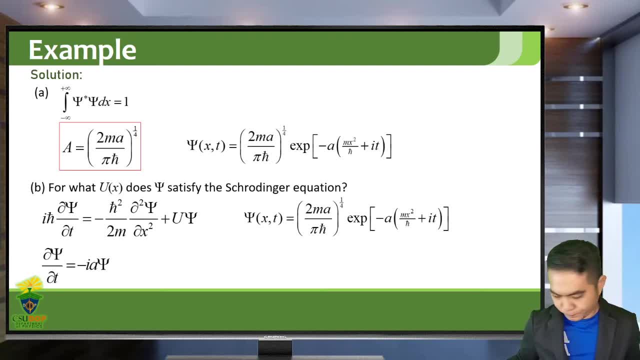 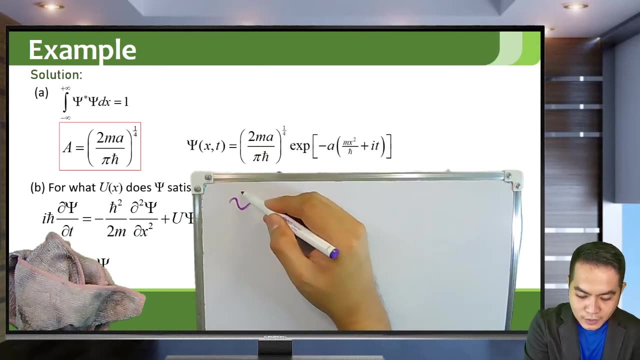 so we integrate with respect to time. so integrating with respect to time, given our psi here, this is our psi. so take note that we can write our psi as a function of x and t. as i will just write this, so it will not be lengthy, i will just write out this constant here as a. then you will have e to the negative, m, a, x squared over, a is equal to a and the answer is negative. um, so that's all for this experiment. so if you want more help, please subscribe to this channel and also like us on social media and also share this video with your friends and also comment on this video if you did, and I will see you in the next video. 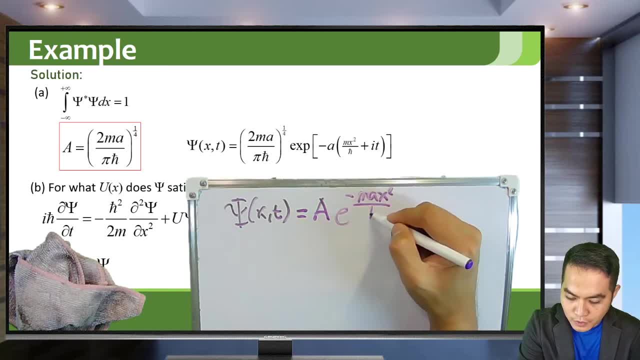 thank you for watching. have a nice day and have a good day and goodbye, bye, bye. x squared over h bar: this is the x component in this exponential and then e to the negative, i, a, t. this is the time component. so if you take the derivative of this, 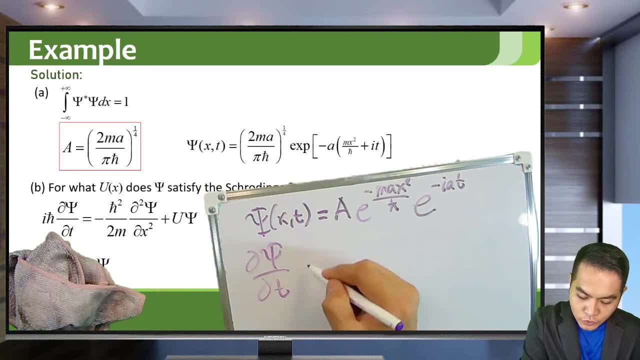 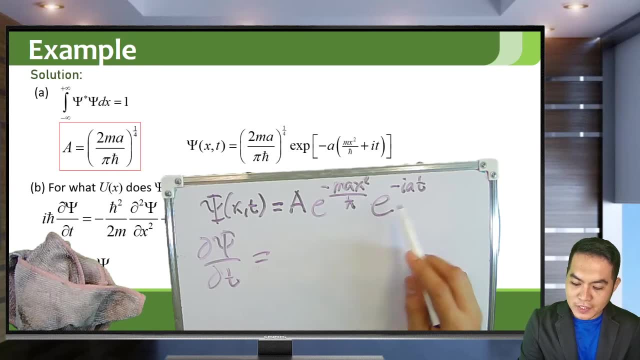 with respect to time. you are actually only taking the derivative of this term here. so what's the derivative of this term? so the derivative of this term is just of any exponential. is e to the? u derivative of? u, the power. so you will still get a e to the m? a. 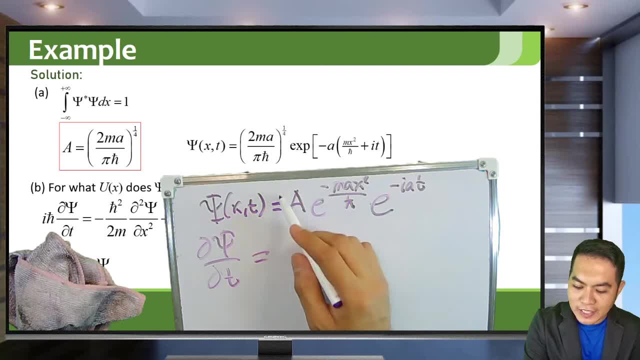 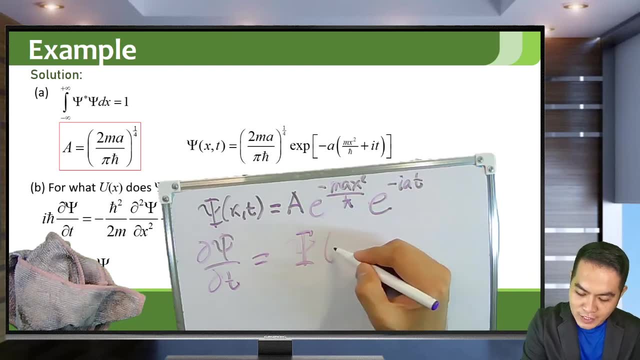 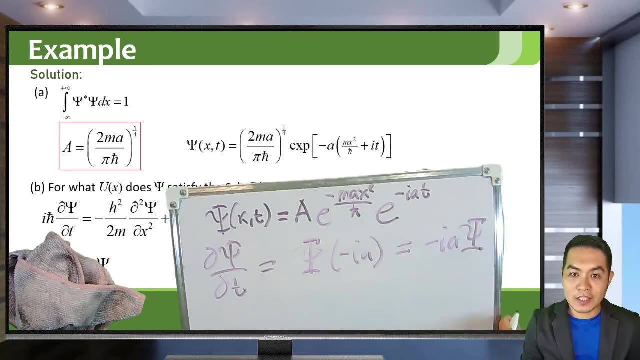 x squared h, bar e, to the which negative i a t. you still get this term when you take the derivative, which is just your psi, and then the derivative of this term with respect to t, which is just negative i a. so therefore, partial side respect to t is just negative i a times psi. 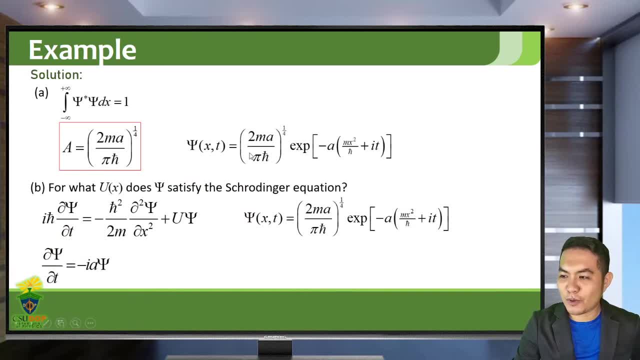 sorry, that one. now you do the same for x. you take the first derivative first and then you take the derivative of the first derivative to get the second derivative, and you will obtain this expression here. so i will just leave the differentiation to you, because it's just. 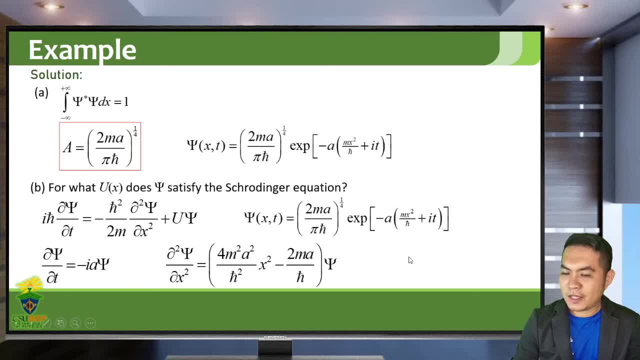 elementary differentiation. there's, no, there's nothing complicated yet. okay, so if you substitute partial of psi with respect to t back to r squared equation here, and you substitute the second partial derivative of psi with respect to x, which is this expression, substitute it back here and solve for u. 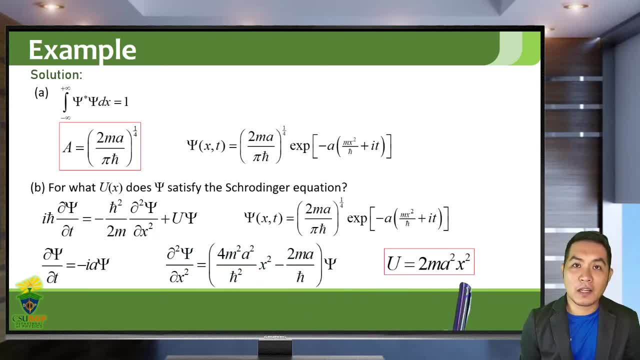 then you will get this result. so i will leave that to you, because that's just simple substitution, simple algebra. so the result is this one. so it's a quadratic, it's a quadratic potential. one, two m, a squared, x squared. where a is a constant, m is the mass of the particle. 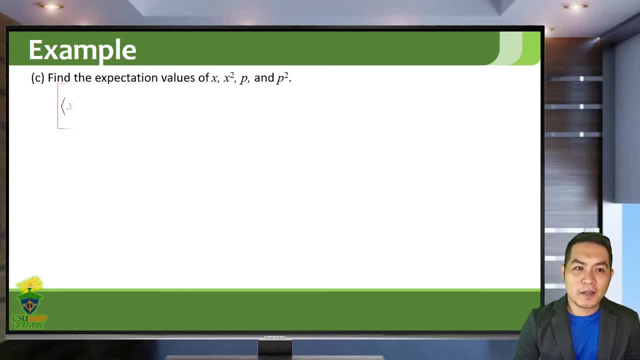 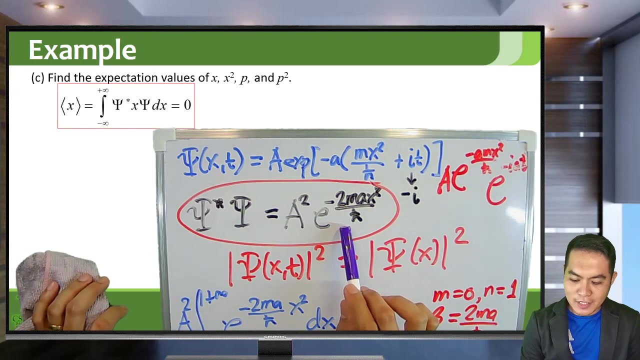 so let's now find the expectation values of x, x squared, p and p squared. so for expectation values of x, we send which x between psi, star and psi, and since our sorry, sorry toist, sorry toist side will just look like this: and this is an even function. so if you multiply, 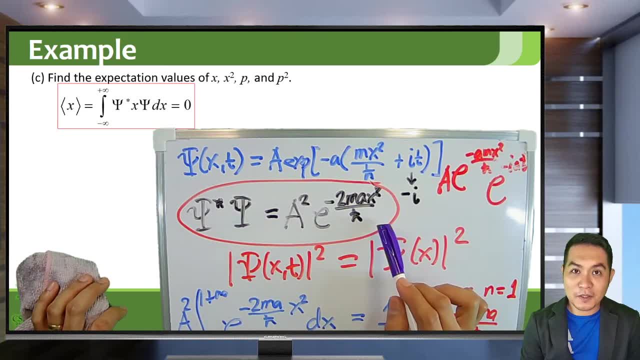 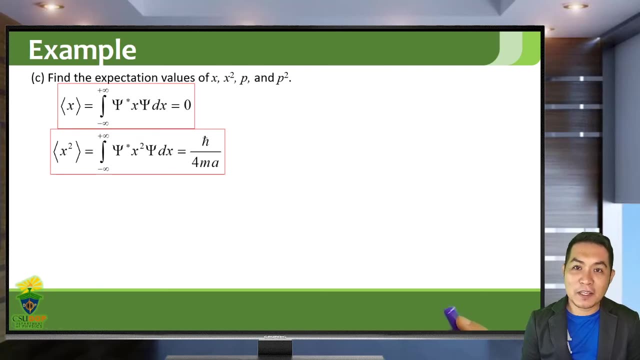 it with X, it becomes an odd function, an odd integrand even limits. that's why it's automatically zero. so it's an odd integrand okay, but not for the case of x squared. for the case of x squared it's now an even integrand even limits. so in 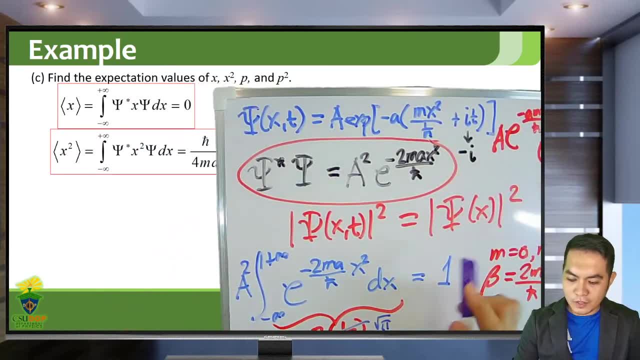 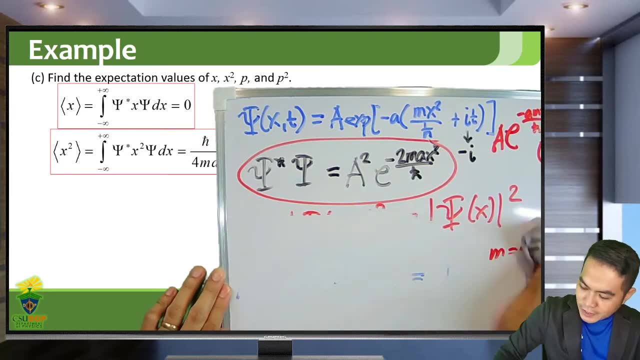 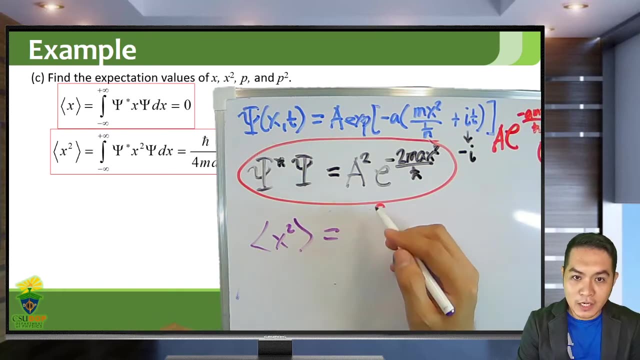 the case of x squared, you will have something like: x squared. in the case of the expectation value of x squared, you will have something like: so you take a squared, I will just substitute a squared later, even though we already obtained the result for this, so your integral will look like negative infinity to. 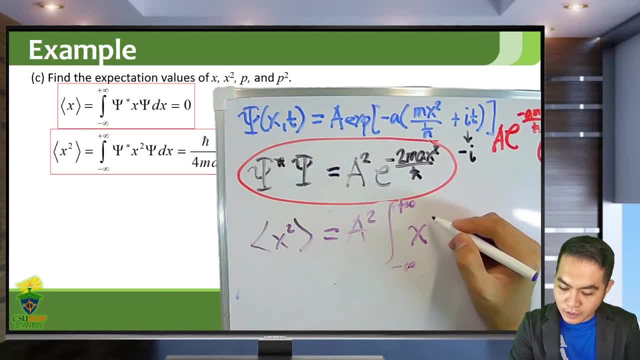 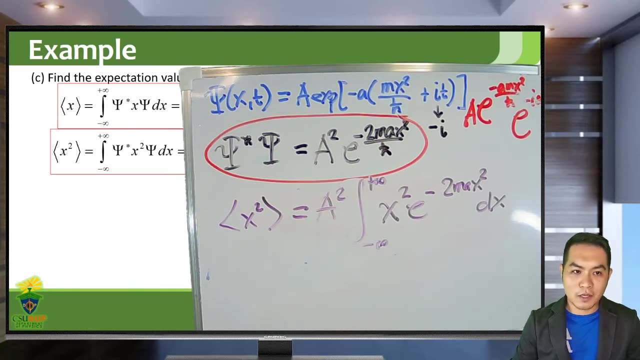 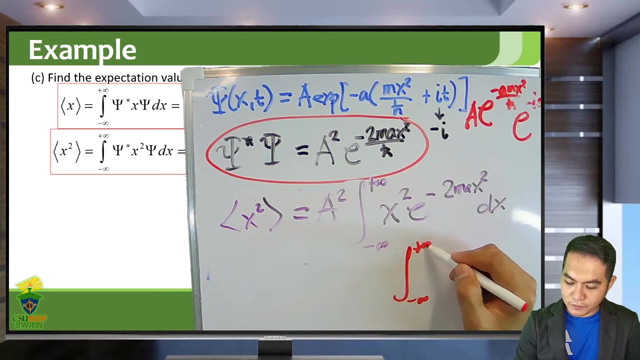 positive infinity of X to the x squared e to the negative 2m, a x squared dx that one. so this integral actually looks like our, the integral formula for the gaussian, the gaussian integral formula before. so in this case, if you will recall, the gaussian integral is from negative infinity to positive infinity of x to the 2m. 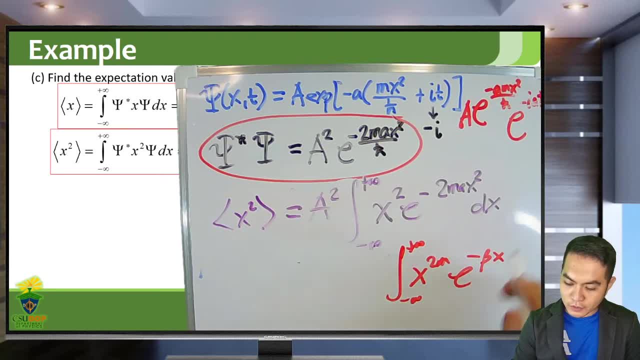 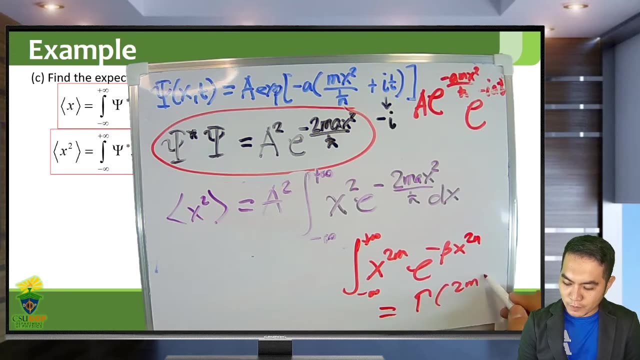 e to the negative, beta x to the- sorry, this should be an h-bar here over h-bar- beta x to the 2n. so the integral, the Gaussian integral, looks like this and it's just equal to the gamma of 2m plus 1 over 2m, over n times the beta to the. 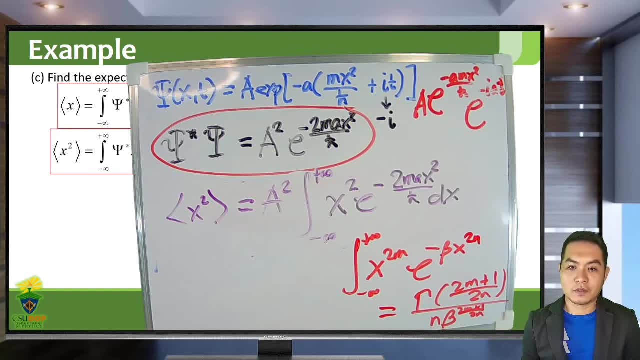 power of 2m plus 1 over 2m. that's our integral formula. so you use that integral formula to evaluate this expression. so from here we see that m is equal to 1 and n is equal, also equal to 1. so you use that integral formula to. 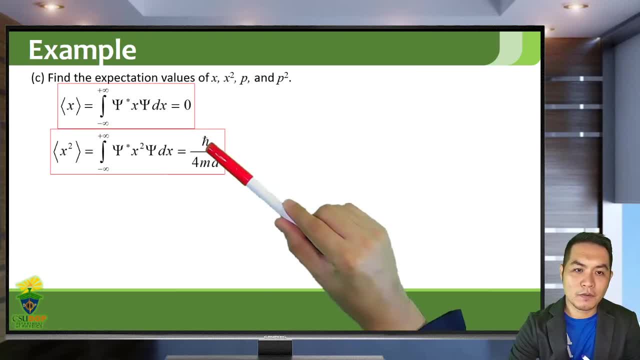 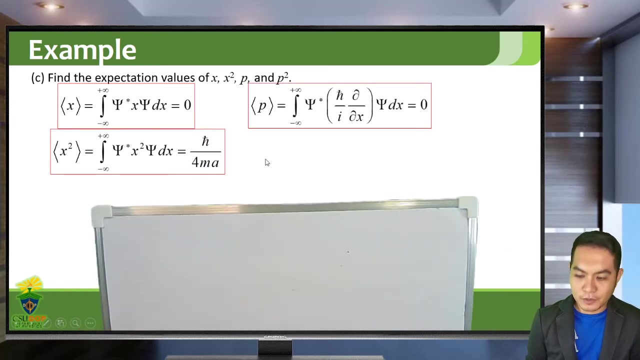 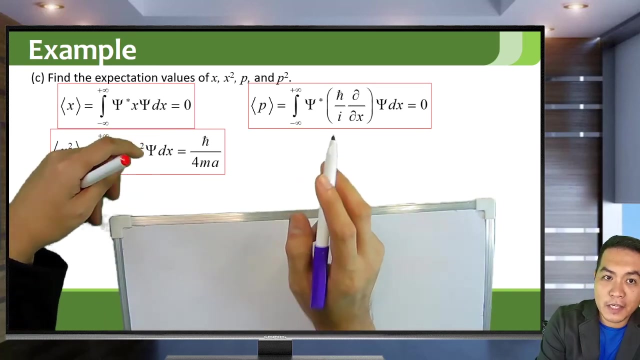 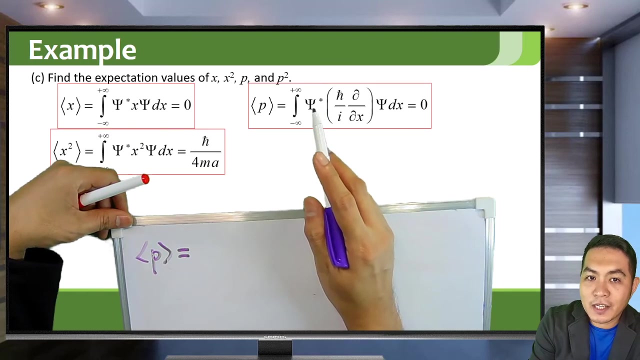 obtain this value, h-bar over 4ma. so how about for the expectation value of momentum? so we haven't yet have any had any example for the expectation value of momentum, so we will try that out first. so this is our formula for the expectation value momentum. so psi star has a term a and psi also has a term a, so I will. 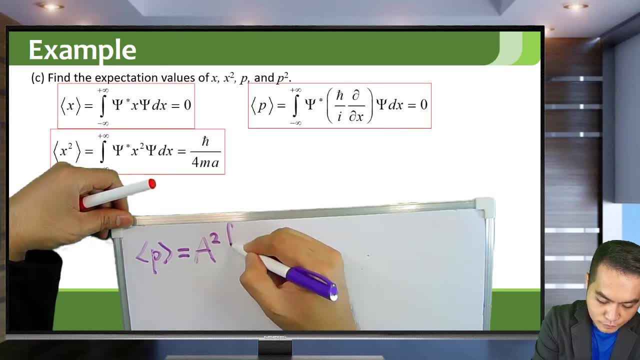 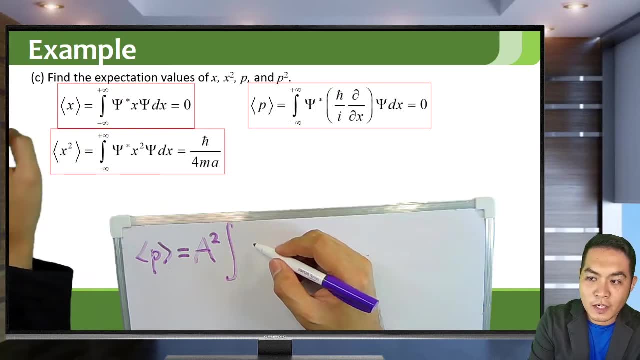 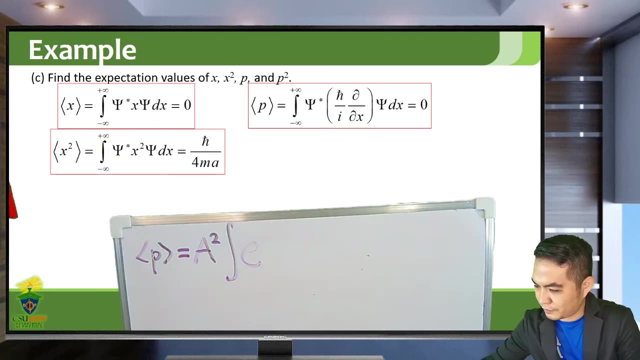 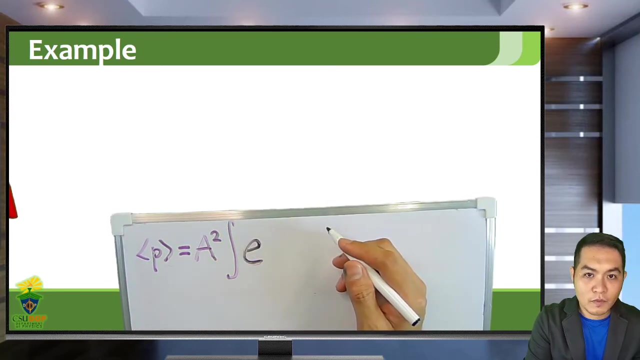 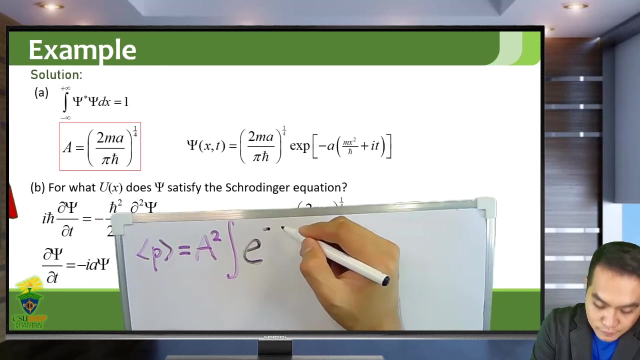 take out that of the integral, the constants, so what's left in the psi star is the exponential parts. so if we take the conjugate, so you will get e to the. I'm just gonna go back to that. I know e to the negative, the ma x squared over h-bar and the conjugate is e to the, so that's. 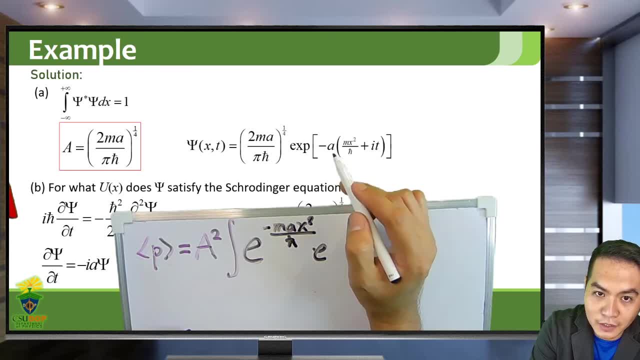 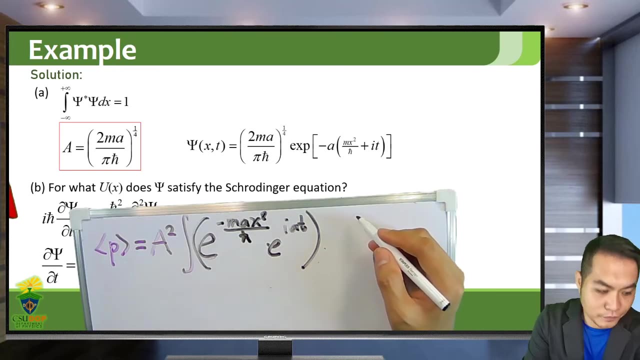 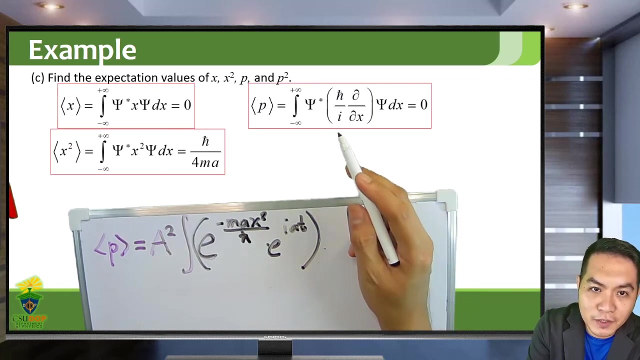 negative a it or I 80. therefore negative I becomes positive I, so I 80. this is what's left of psi star. I already took out the constant normalization, constant a here, and then we have from our formula our momentum operator, so I will take out h-bar over I outside. so there, 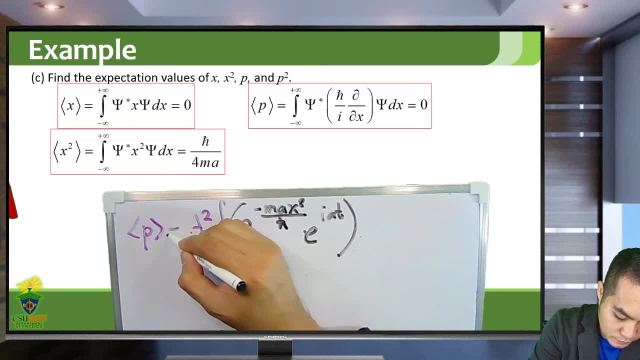 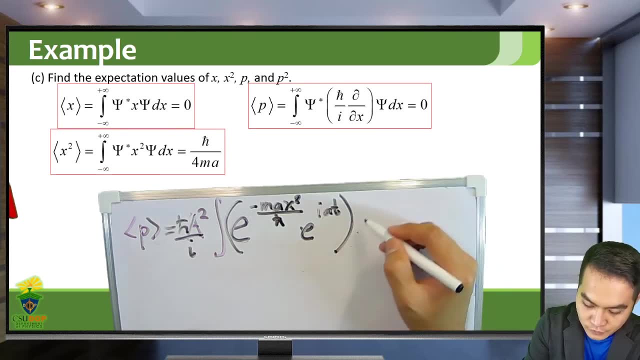 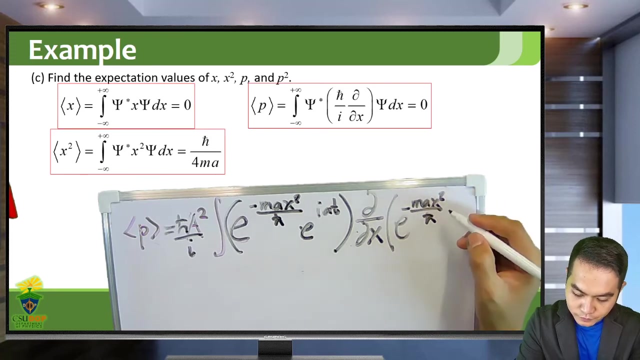 will be an h-bar here, sorry- over I, and then I will the partial derivative. with respect to X, the differential operator will act on what's left of this quantity, here, psi. so what's left is the original version, not the conjugate. so you have e to the negative, ma x squared over h-bar, e to the negative, I 80. so 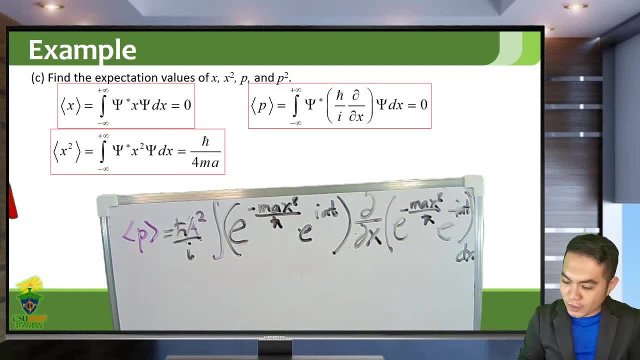 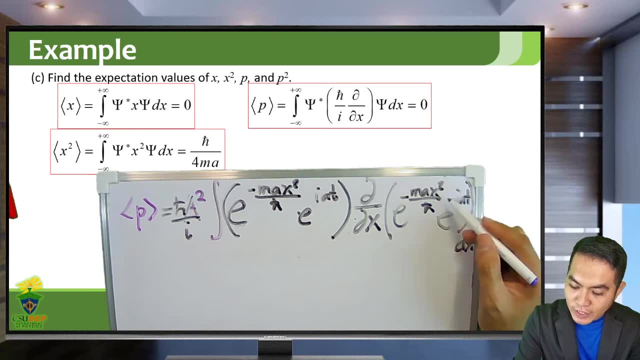 there's a DX here, okay, okay. so since we are all only differentiating with respect to X here, then we can actually take the time component here out of the differentiation and multiply it with this and you will notice that something like this one and this one will just be equal to e to the 0 or 1. so the multiplication of e to the 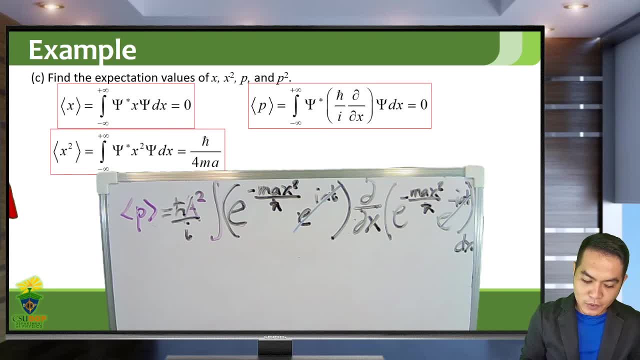 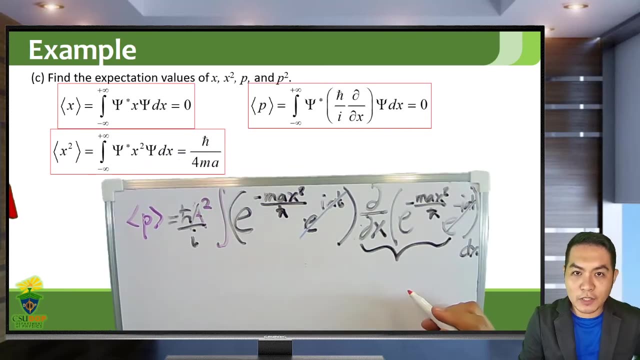 I 80 and e to the negative. I 80 is just 1, so in order to evaluate this, we first need to know what is this differentiation with respect to X? so the differentiation of e to the u, and this is just e to the u. the differential of u, so our u here's negative. 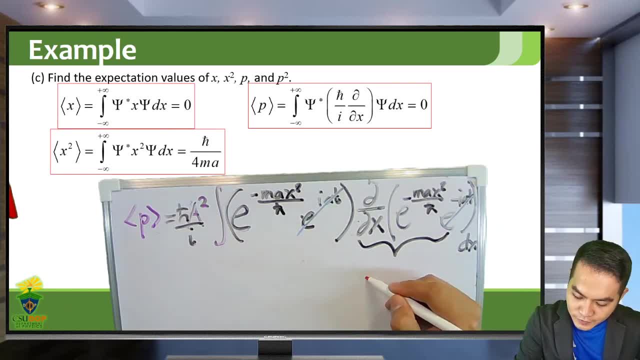 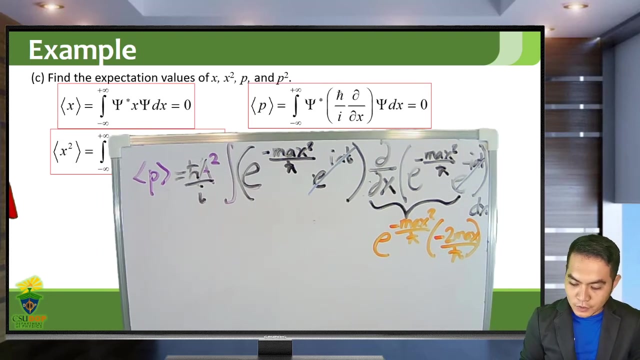 max squared over h-bar. so therefore this differential is just equal to negative max squared over h-bar times the differential of m a x squared over h bar, which is x squared. so you have negative 2m ax over h bar. ok, so the differential operator has already been applied. so this term here and this: 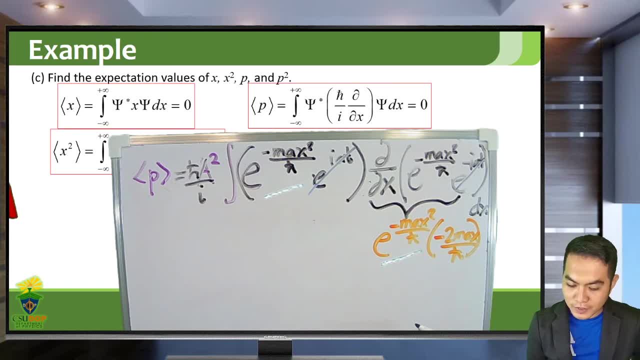 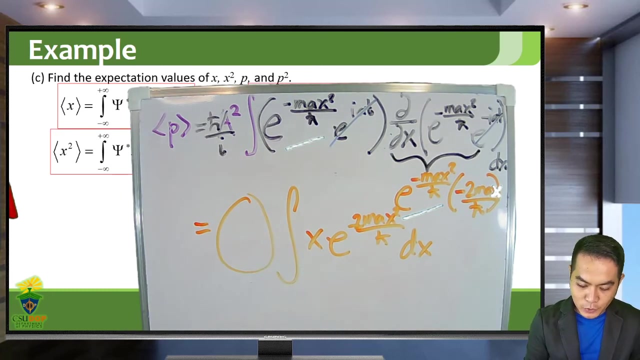 term. here you can add their powers and we are left with X. there's an X here. so in the integral you will some- you are in the evaluation of this expression- will have some constants out to the integral, and then the integral of X, e to the negative ma, so sorry to ma x, squared over h bar DX, and again, since you are, 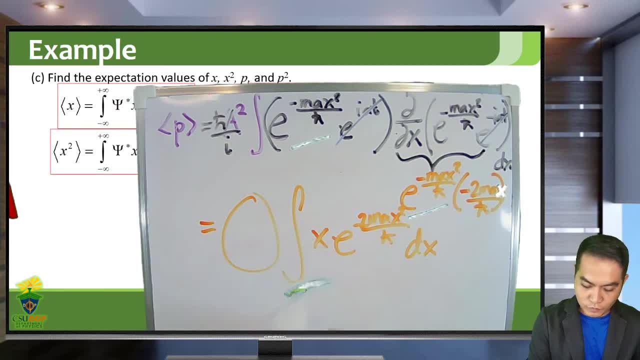 integrating from negative infinity- sorry, negative infinity- to positive infinity, even limits. but the integrand is, since this is just X, an odd function. integrand is odd and even the limits are even. then this one is a right. so this one is a right, so it only has some. 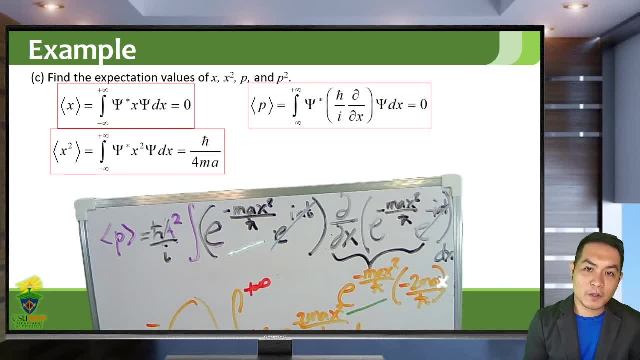 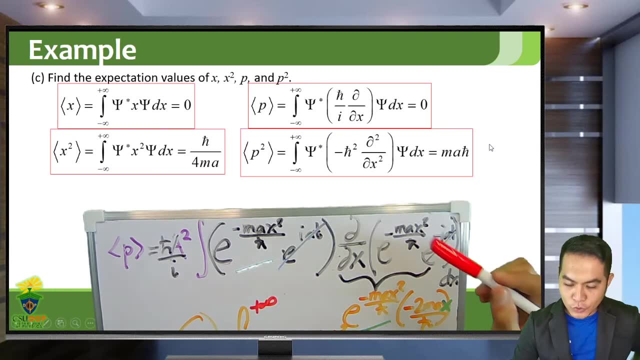 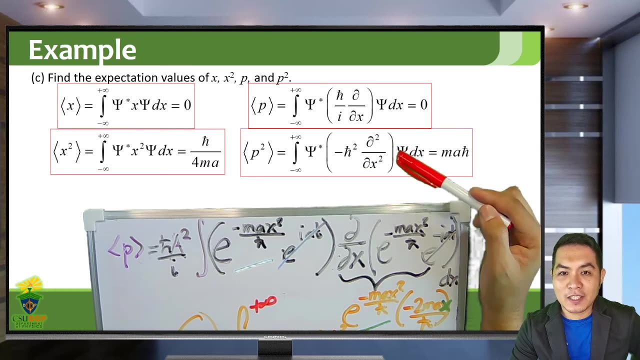 cuerbooks here, and then this is well, we have this one right here, and then this element right here and this one is a right. so at the end of the expression we will have a vector value of 0 when the h bar squared and i squared. i squared is negative one, so that's negative: h bar squared. 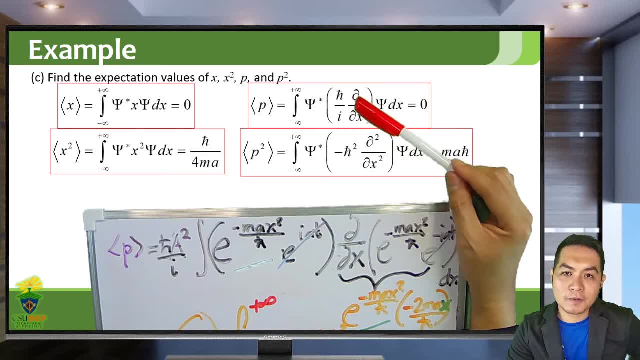 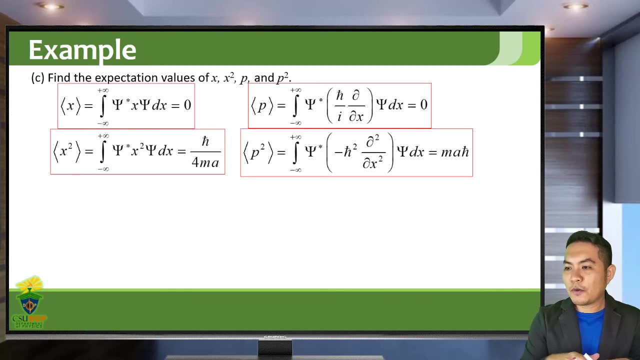 and then if you add the derivative twice, then you have the second derivative. so you need to find the second derivative of psi first before you evaluate this integral. so you do that, i will leave that to you and you will get a value of ma h bar. okay, so you now know the expectation values. 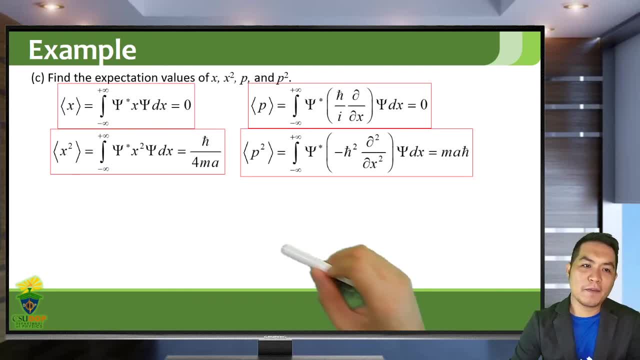 of x, x squared, p and p squared again. the meaning of this expectation value is that the values of x- there are values of x that's positive, there are values of x that's negative. that's why the average value is in the middle in zero. the same is true for the expectation value of. 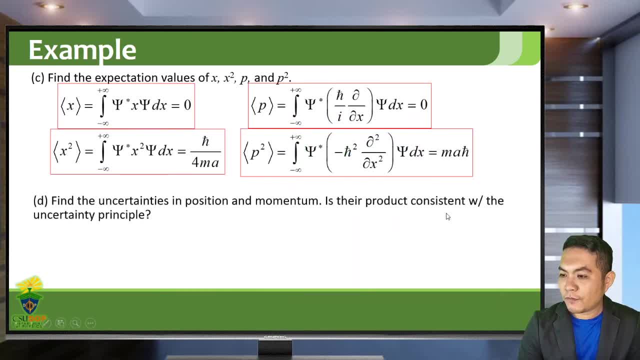 p so find the uncertainties in position and momentum and is their product consistent with uncertainty principles. so therefore we use the uncertainty formula for x. it's just the expectation value of x squared, minus expectation value of x squared. so this, since this is zero, it's just the square root of the. 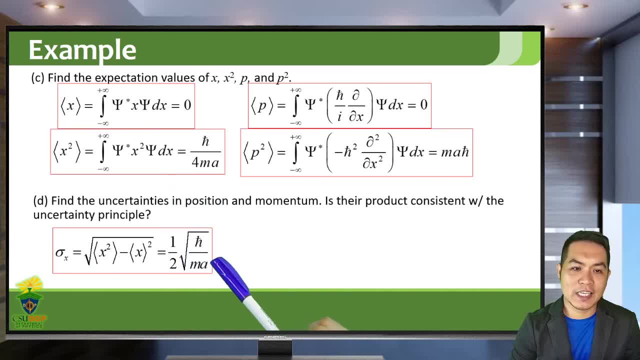 expectation value of x squared, or square root of this term here, which is just this one one half square root of h bar over ma and the same for p. you will get just the square root of this, which is square root of ma h bar, since this term is zero. 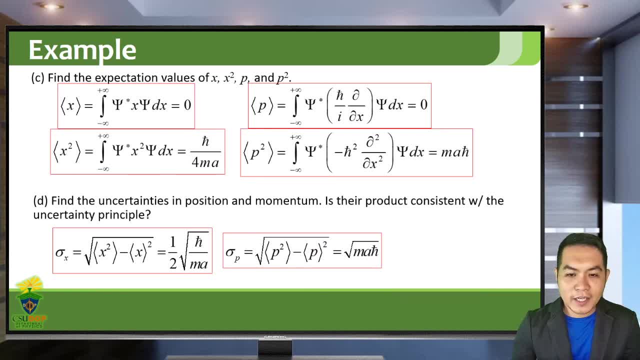 so to check if we, if the uncertainty principle is not violated, then we use this equation and check: is this true? is their product or are the? is the product of their uncertainties greater than one, greater than or equal to h bar over two? so we have a question mark there, because 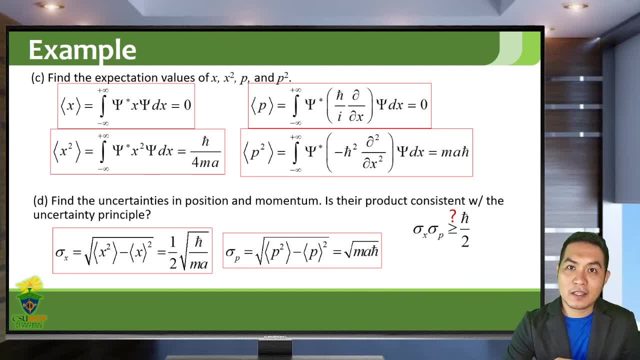 we're trying to prove if- uh, it's, if- their product is consistent with the uncertainty principle. so if you multiply these two terms here, you will actually get a value of h bar over two, which is consistent, because this is greater than or equal to h bar over two. so it's equal to h bar over two. so the product of their 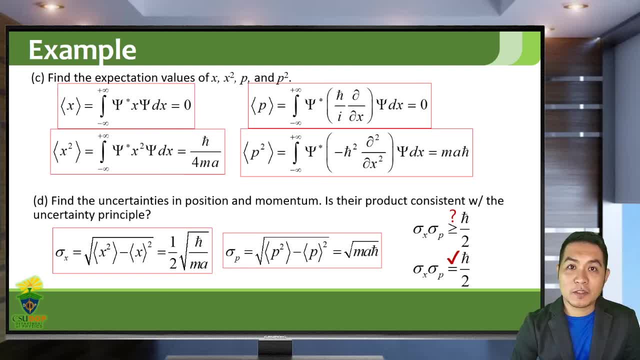 uncertainties is uh consistent with heisenberg's uncertainty principle. so it's, it doesn't uh violate the uncertainty principle. so we're trying to prove if the uncertainty principle is consistent with the uncertainty principle. okay, so this is the generic problem for in quantum mechanics. so you, you will have a normalization problem. you find the expectation values, you find 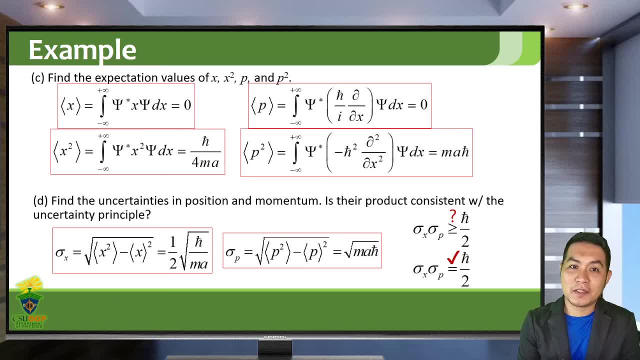 the probability you find the potential energy corresponding to your uh state or your wave function. but there's still one problem that we haven't uh solved uh yet, and that is the problem that we haven't uh solved yet, and that is the problem that we haven't uh solved yet, and that is 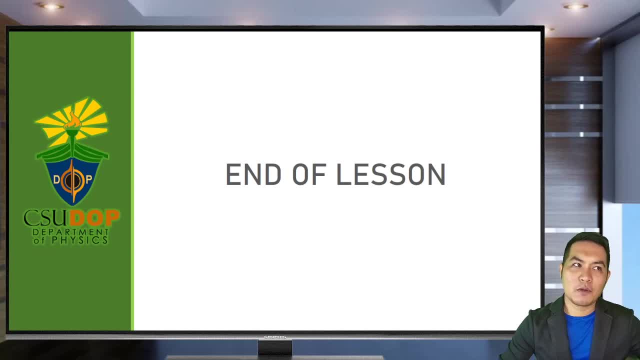 the problem that we haven't uh solved yet, and that is: what if you are given the initial wave function? what if you are given the initial wave function? what if you are given the initial wave function and you are asked to find what's the wave? and you are asked to find what's the wave? 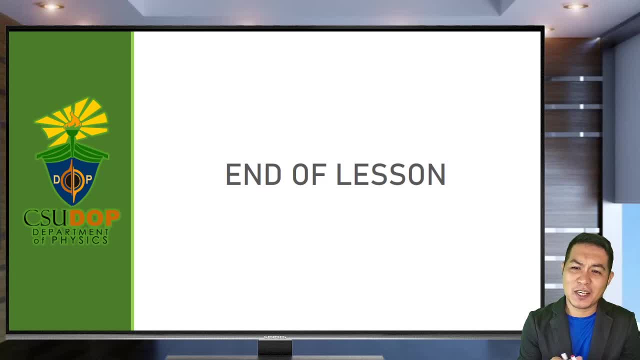 and you are asked to find what's the wave function at any time. t function at any time. t function at any time. t psi as a function of x and t. so how do you psi as a function of x and t? so how do you psi as a function of x and t? so how do you do that? 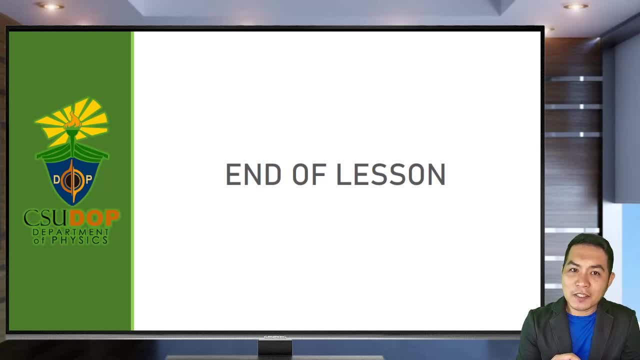 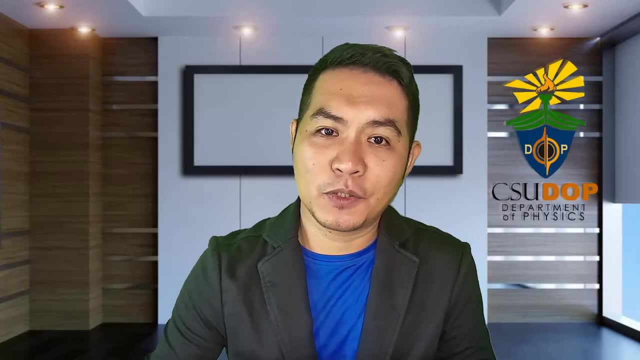 do that, do that so, so, so the answer to that, the answer to that, the answer to that question will be question will be question will be discussed, discussed, discussed in the next chapter in chapter two, in the next chapter in chapter two, in the next chapter in chapter two, where in we will discuss about the time. 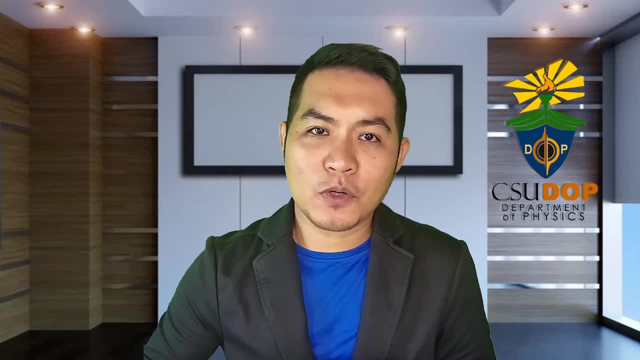 where in we will discuss about the time, where in we will discuss about the time. independent school equation. independent school equation, independent school equation. so we'll try to solve, so we'll try to solve, so we'll try to solve. given the initial wave function, we will. given the initial wave function, we will. 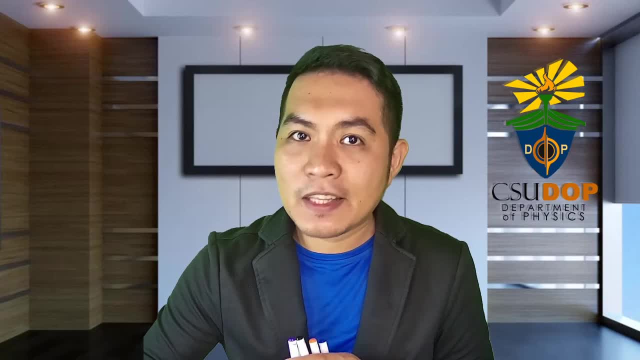 given the initial wave function. we will try to get the wave function at any time. try to get the wave function at any time. try to get the wave function at any time. t for different types of potential. t for different types of potential. t for different types of potential energy. so that will be our lesson. 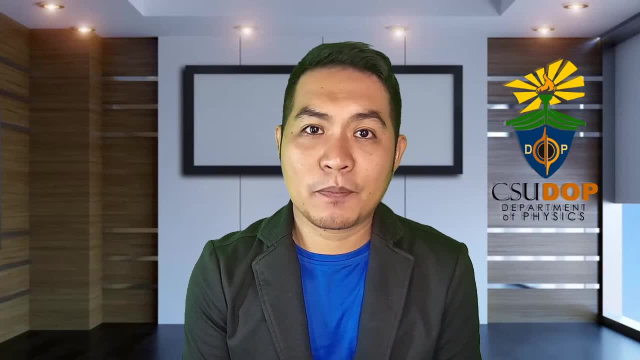 energy. so that will be our lesson: energy. so that will be our lesson for the next chapter. and this ends the for the next chapter. and this ends the for the next chapter. and this ends the chapter on the wave function. so so far. chapter on the wave function. so so far. 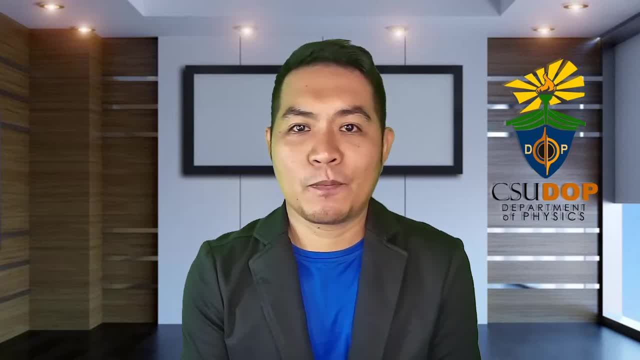 chapter on the wave function. so so far, we have discussed some basic properties. we have discussed some basic properties. we have discussed some basic properties of the wave function. but when we go to of the wave function, but when we go to of the wave function, but when we go to chapter 3, we'll now formalize our wave. 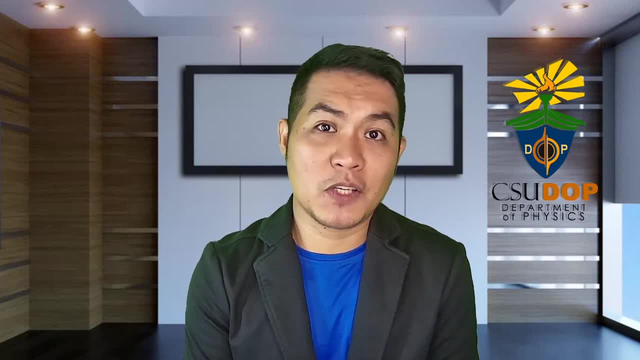 chapter 3. we'll now formalize our wave chapter 3. we'll now formalize our wave function function function such that it's not just a wave function, such that it's not just a wave function, such that it's not just a wave function in position. 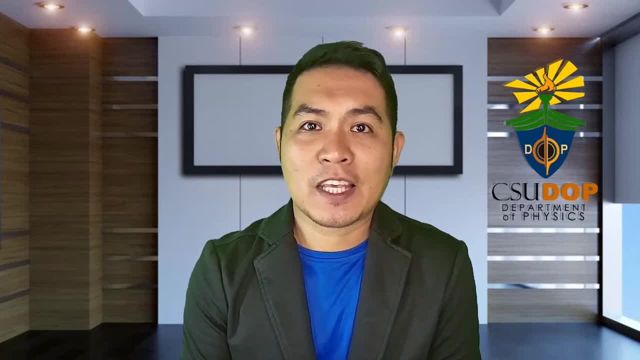 in position, in position, position space, in fact, the wave function, position space. in fact, the wave function, position space. in fact, the wave function can be, can be, can be formulated in position space or in energy, formulated in position space or in energy, formulated in position space or in energy space or in momentum space. 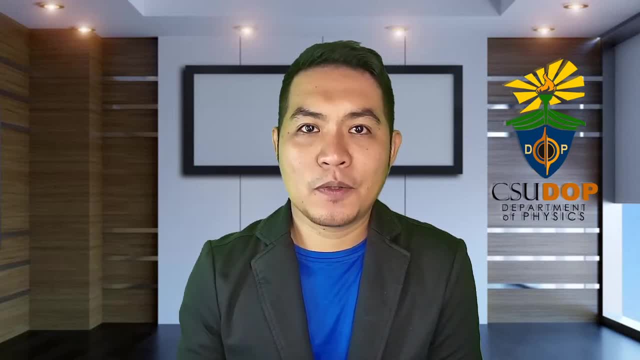 space or in momentum space, space or in momentum space. so that's the end of this chapter and i so that's the end of this chapter and i so that's the end of this chapter and i will see, you, will see, you will see you at the start of chapter two, which is on. 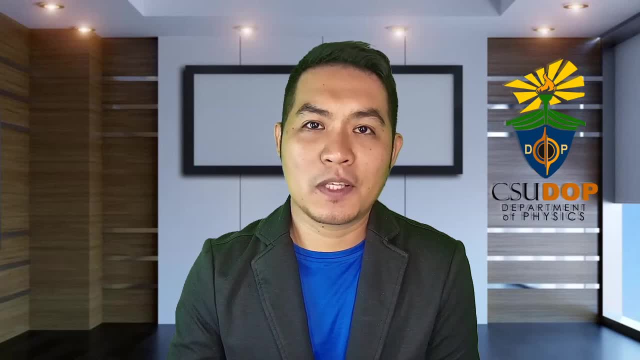 at the start of chapter two, which is on at the start of chapter two, which is on the time independent: the time independent, the time independent screwdriver equation. so i will see you, screwdriver equation. so i will see you, screwdriver equation. so i will see you next session. next session. next session.